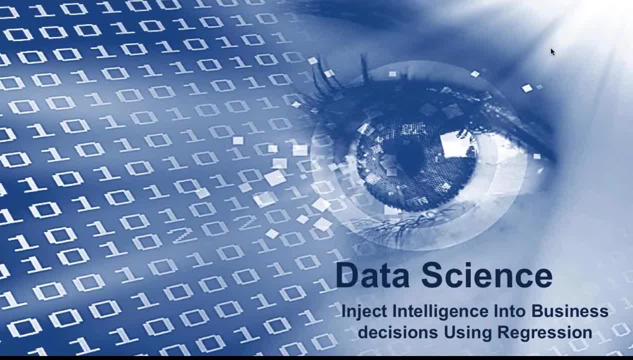 Hi there, good morning, good evening to all of you from different parts of the world. My name is Anirudh Kala and I'll be taking this webinar on Logistic Regression. Alongside Logistic Regression, we'll also cover few basic concepts on R and what is data mining and machine. 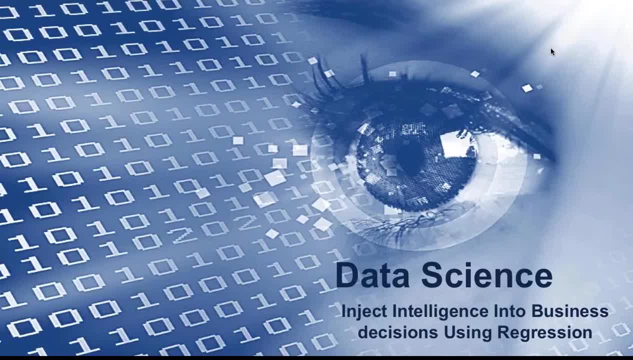 learning, what is the data life cycle in a machine learning paradigm and how exactly do we productionize a machine learning system? Okay, so let's start. So, basically, this particular webinar is going to focus on how data science is changing the behavior of industry. Second, what is a data? 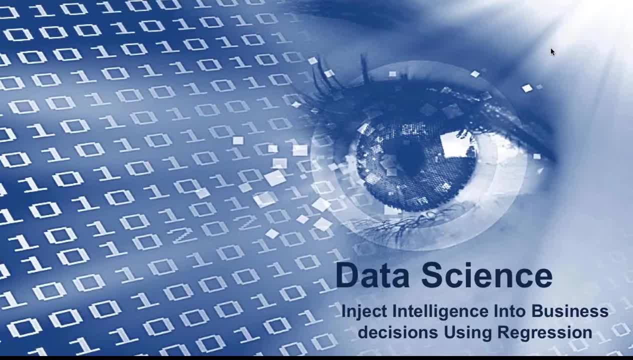 science project life cycle in a production environment and thirdly, the tools and the algorithms that constitute this new environment called data sciences. I'm going to pick up one and Gartham and we'll see how exactly do we implement it with a real-life case. 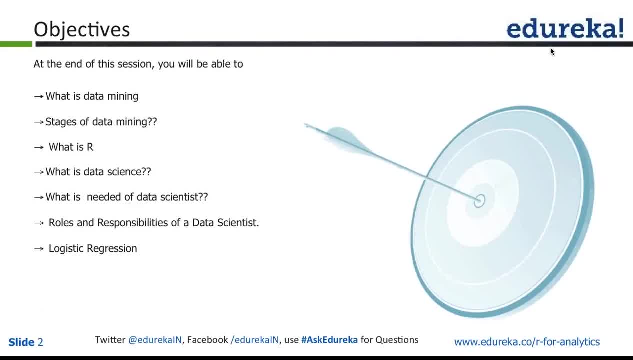 study. okay, so here we go. so objectives of this session would be that, after the session, you should be, you should be- knowing what is data mining, stages of data mining, what is our, what is data sciences, what is needed of a data scientist, roles and responsibilities of a data scientist. and 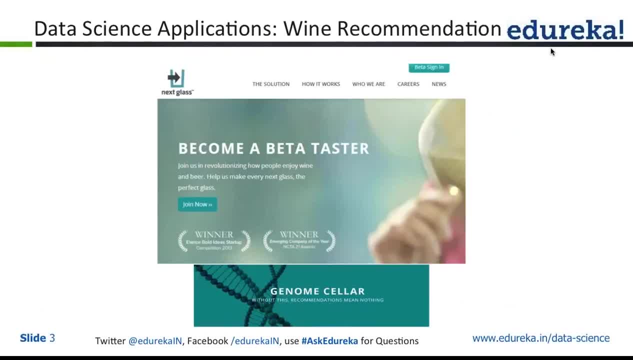 last but by no means the least, the logistic regression exercise. so the actual exercise that we're going to do today is going to focus on logistic or logit, regression. so data science, applications, wine recommendation: well in in, specifically in France, and in the northern coast, the eastern coast of North. 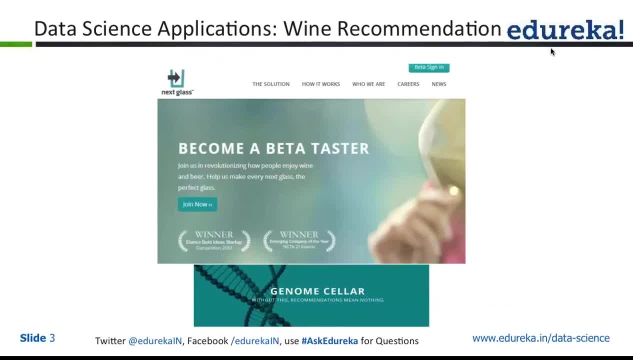 America you'll find a lot of people who have a career which relates to wine testing, and those wine testers are really highly paid guys. so they taste and they'll figure it out if the the taste of wine is good or bad. but based on that they also can they also tell us what kind of people would like that kind of 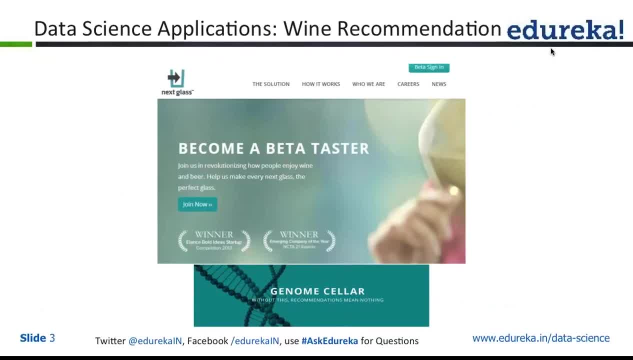 fine. so data science is helping figure out who are the set of people who would like a particular taste of wine. and let's say, if I like a wine of quality X, what are chances that I'll also like the wine of quality X? what are chances that I'll also like this wine would also be helpful to me. 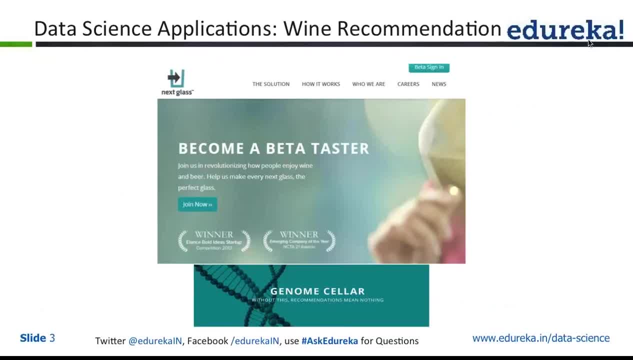 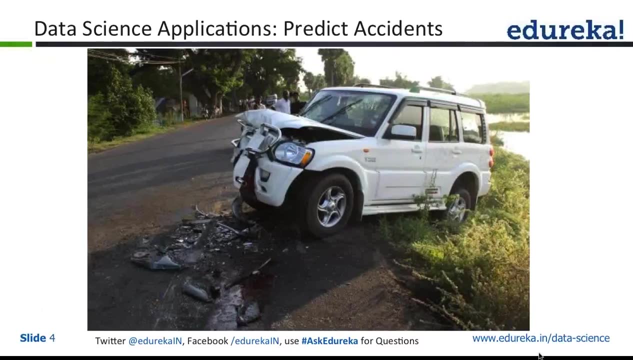 wine, of quality or taste, why. and they are making a recommendation engine which helps in which helps in figuring out what to be served to whom. well, we also use a data science to predict accidents. can we actually do that? is there a real causality or a correlation that can help us predict accidents? well, the answer is a. 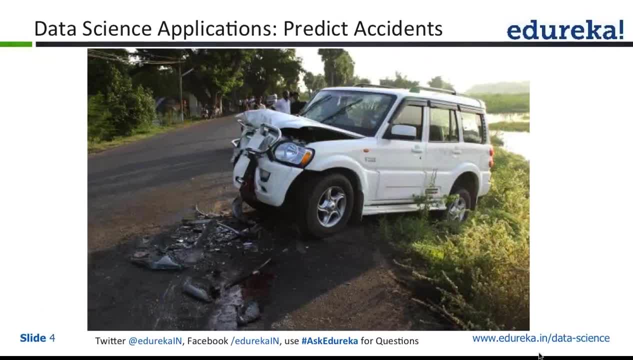 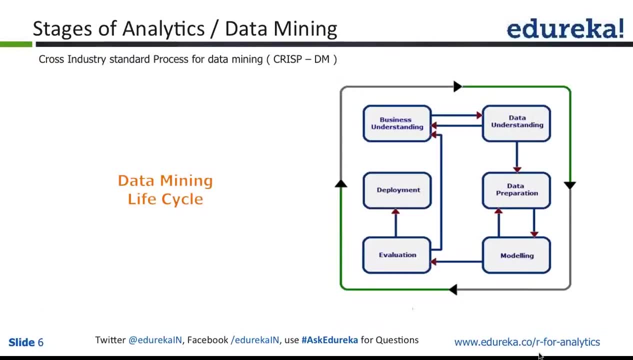 yes, we can do that, and that is exactly the exercise we're going to do today are using logistic regression, so just wait for that. stages of analytics and data mining. so, basically, in a production environment, there are few stages that you need to be very careful about now. this is not. this is not a pretty much. 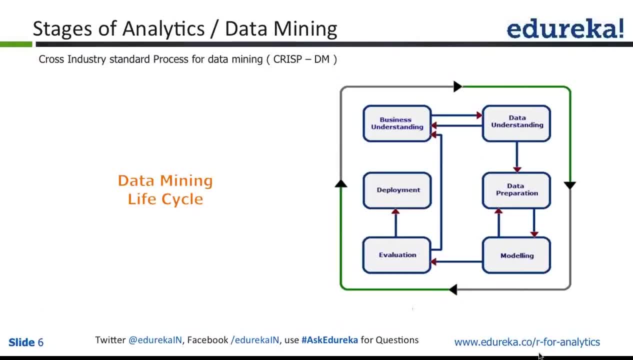 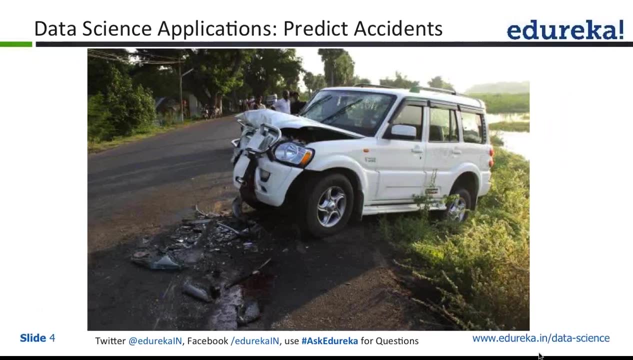 similar to a software development lifecycle. the idea is same. the idea is: you know it is something and you evaluate it, and then you, you know, finally productionize it. but these stages are different. so one stage which is really important is data understanding. so, for example, the case 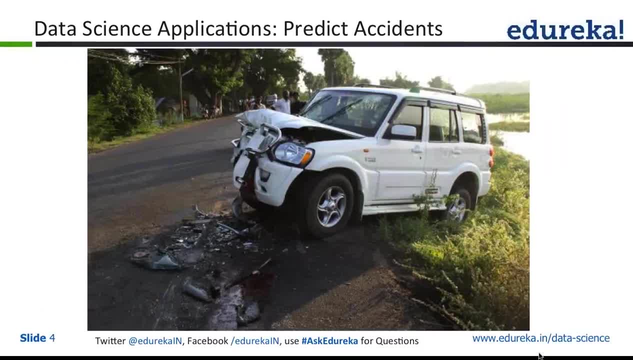 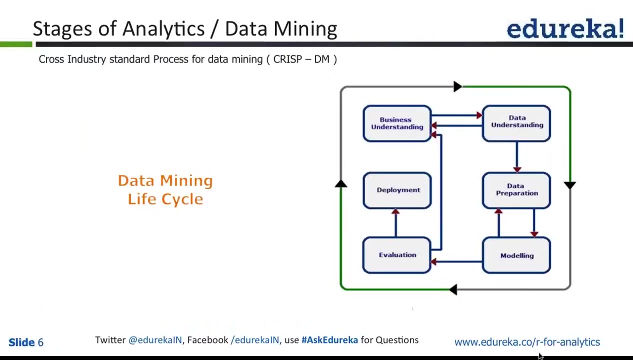 that I was discussing with you on the accidents prediction. we actually need some kind of a domain knowledge also to understand. can that really be a possibility to predict? well, in in scenarios like epidemiology or algorithmic trading, where you can figure out if a, if a particular stock is going to go up or down, and point one seconds. 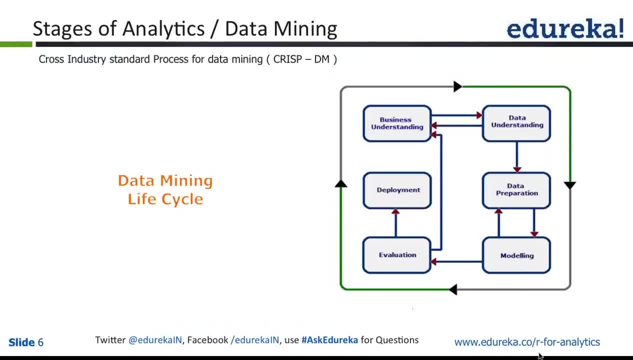 then you can do, or you can sneak out, some arbitrage in that particular trading. so domain experience are the data understanding part is really crucial, because if you don't know what exactly is lying under the hood, then you cannot figure out how we can use that data. 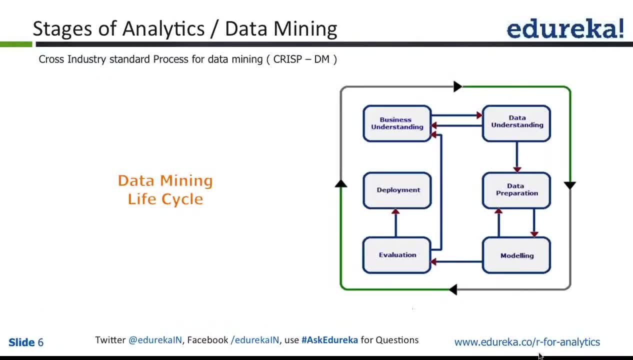 now think of an example where you're supposed to figure out that offer that you're giving to a particular person. will you read that offer or not? then you need to know what are the habits of the purchase habits of that person. then you also should know what domain puts in where. so basically, do you know the? 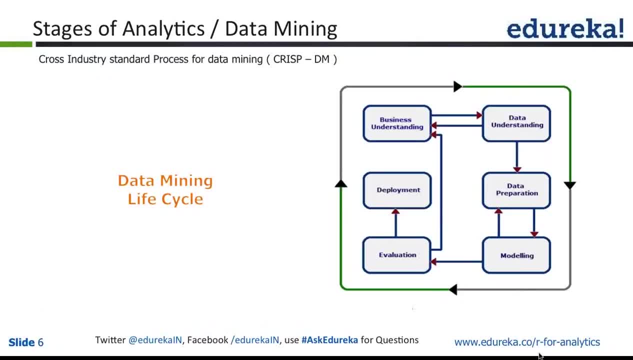 retail supply offer, the retail supply chain of a particular product. do you know the inventory of that particular product? do you know the market of that product? do you also know the customer segmentation for that product? all these questions can be answered by someone who comes in with the domain experience on that particular. 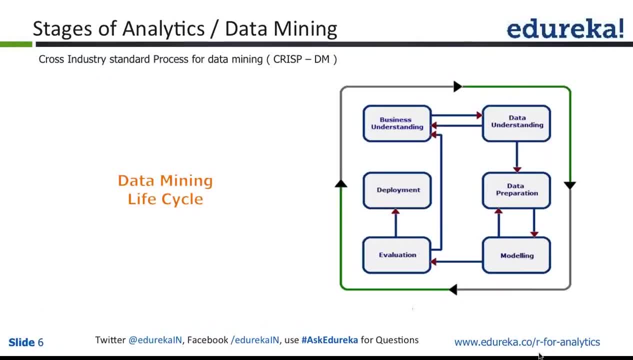 domain and thereby gives us the understanding of the data. the next is data preparation. now we already have the data, then why the hell do we need to have a data preparation? well, a data preparation is is something like where you figure out the hidden data points. now think of it. I mean, think of the same. 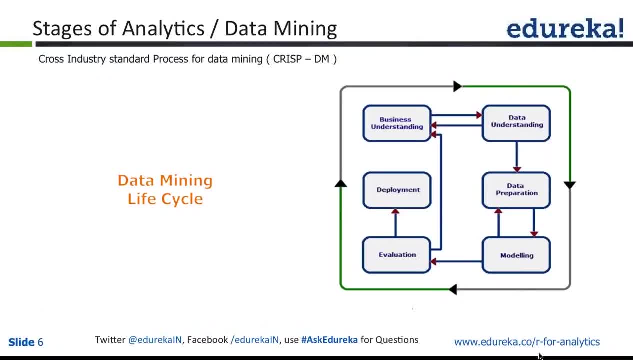 example I just gave, where you need to figure out whether a particular person will accept an offer or not. and let's say you were given the entire history of his custom office purchases in the last one year. so let's say you have an offer on honest on a soap, then figure out how many number of soaps, how many. 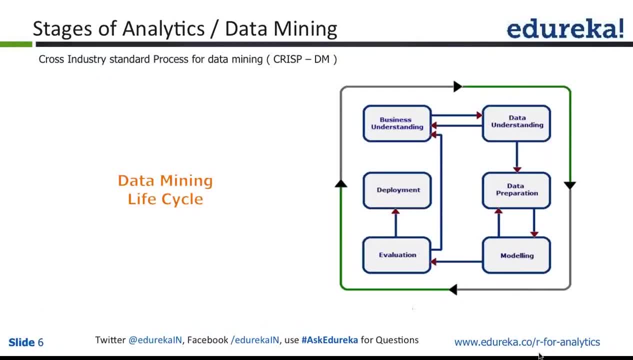 brands, rather for a for soaps has this person bought in last one year? now that's a different column all together. now getting that column can help us figure out if this person is brand savvy or not. so basically using the same data set, you figure out some more attributes about that person. that is called a data. 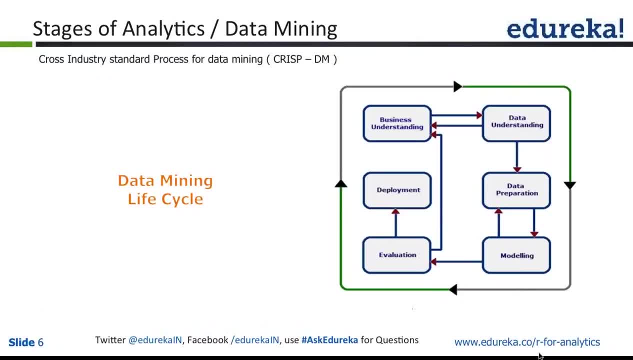 preparation plus cleaning the data is also part of data preparation exercise. also, putting data into different formats forms you have to change something to a number or something into a character. so all that data cleansing and data massaging part happens in this data preparation stage. then comes the stage of modeling. now what is modeling and 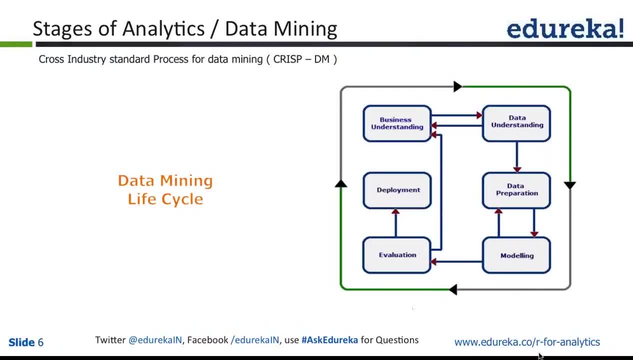 why the hell in the world? we call it a modeling step. so basically, what we do is we create analytic, analytical models, which are nothing but state-of-the-art algorithms that are known in the in the in the industry of data sciences. so logarithms could range from big, complex, neural 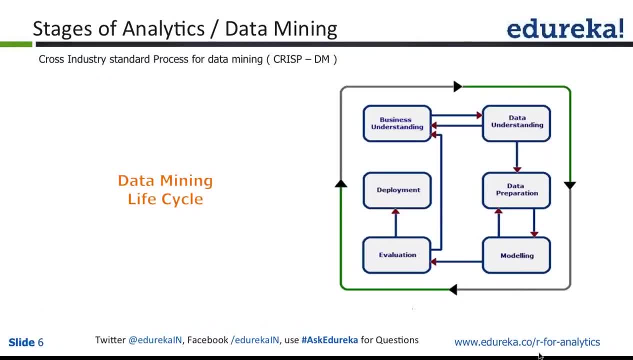 networks to as simple as you know, regression and all these algorithm constitutes- I mean the algorithm that you put on on a data. it could be one, it could be mixture of multiple models, the multiple algorithms that'll create a form, something as a model, and that model is something you can use for building. 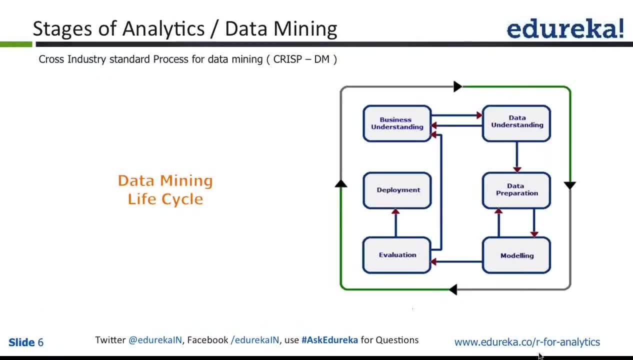 some prediction, doing some recommendation, doing some target analysis and once you have the data model prepared, you test it or you evaluate it. so, basically, you test it on the data set you've not seen so far and then you evaluate the predictions of the model with the actual values of the column. 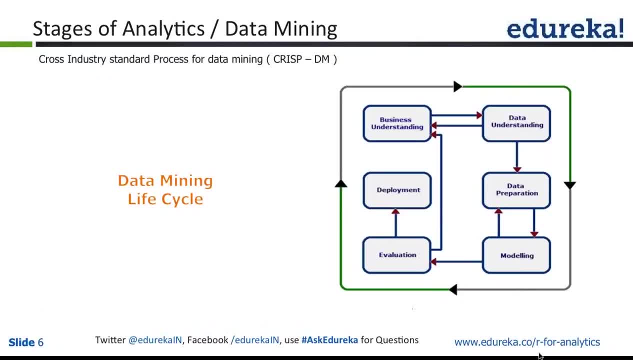 that you're trying to predict on in the evaluation stage. if everything is fine, you go to the deployment stage. if your evaluation criteria is not meeting up to up to the expectation, then either there's a problem with your model or is a problem with your data preparation, or you've 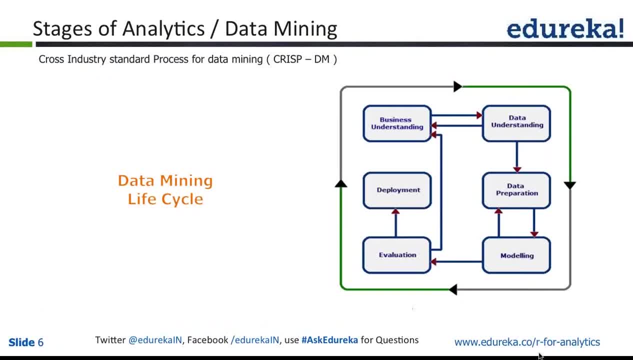 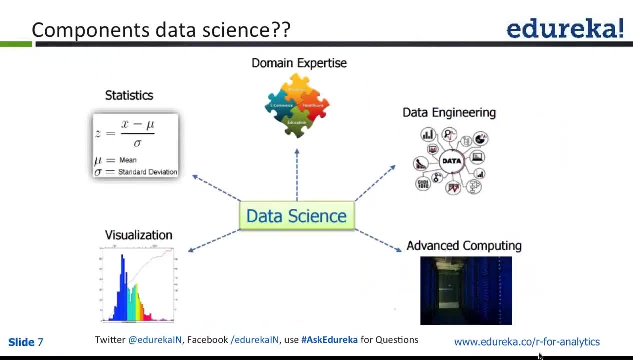 not got the business understanding part correctly, so you go back to business understanding again and see if it's not being sense with the output that you have gone from this entire exercise. if everything is fine, we go to the department stage. well, the components of data science are: 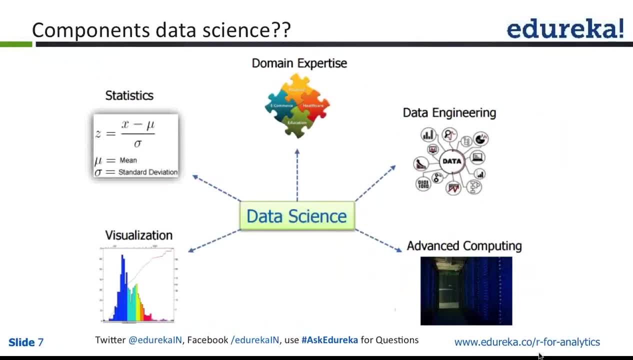 by the way, in case you've got any questions, we'll have a session post. you know I complete all my stuff just for the Q&A, so if you've got the question, just write it down. I'll take it after the class. so there are five very basic and I would say it's not in fact the components, not. 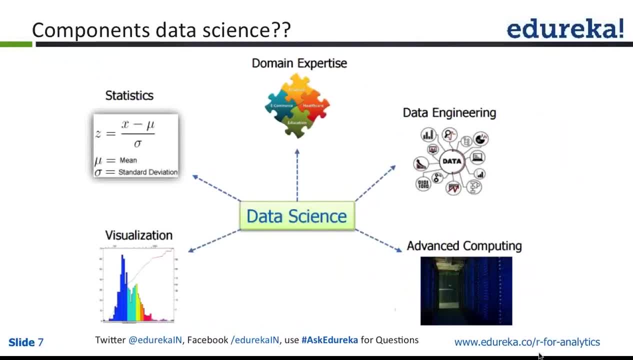 the other pillars. if you miss out on one, you actually miss out on the rest four. so we can start with data engineering now. what is data engineering? I mean, it could be. is it something similar to what we've been doing in the ETL or the extract transform load? 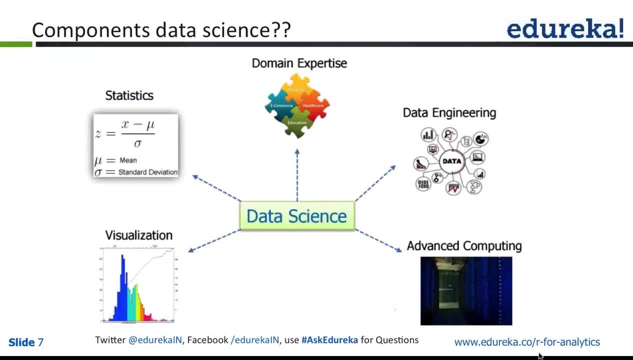 paradigm or something similar to the BI, the business intelligence. well, somewhat that is, and that is because we still treat the data the way we've been feeding it, just that we massage it in a different fashion. we might not put into facts and dimensions, we'd rather put into the. 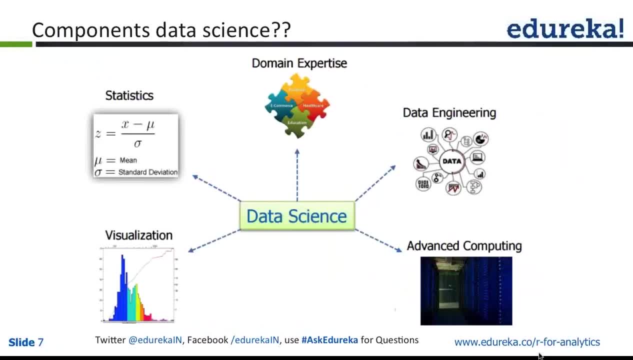 format. we are, we want to, you know, we want to rent on. then there is advanced computing. well, I am sure you guys must. you guys have heard of something called as Hadoop, which is currently the most popular framework for advanced computing. rather, it's not advanced company, to be honest, it's. 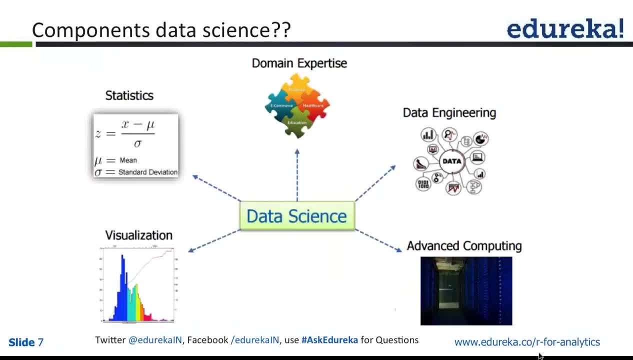 more precisely parallel computing. so parallel computing is like when you've got a task you divide into parallel runnable modules and you put it on something like Hadoop or Spark, which is the new you know buzzword in the market, and do some really advanced computations which were not possible previously or they used to take a. 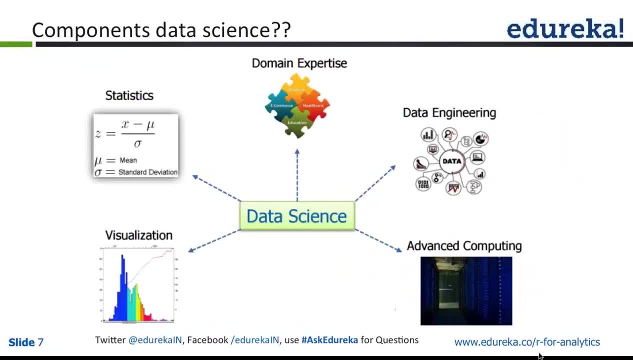 lot of time. the third part is statistics. so statistics plays more than an important role. I think it's the heartbeat of analytics, it's the heartbeat of data science. everything that we do relates to statistics. so if I say algorithm, I don't really mean the algorithm that you 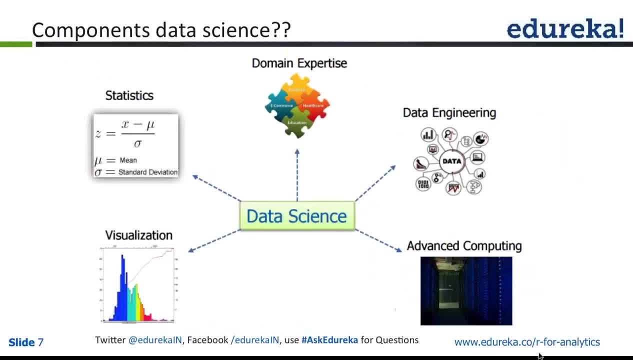 probably would have- would have heard of while doing a course on data science structures, because that's more of a data management algorithm where you manage the data in such a way that the retrieval and their sorting and their insertion is pretty optimized. over here we are trying to figure out something statistically, so all the algorithms that we run they are 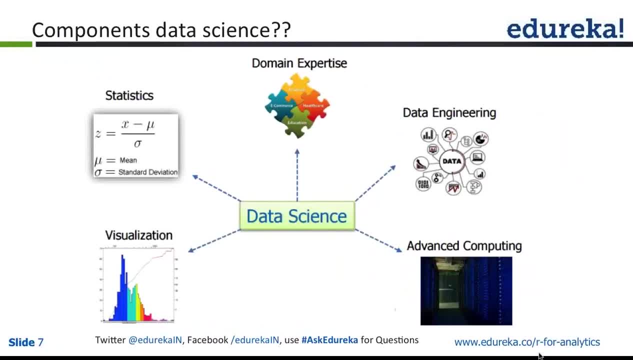 statistically proven. in fact they are. they come up from the branch of statistics called statistical learning, then visualization. well, of course, whatever we do, we need to present in such a fashion that it makes sense. so with data sciences we go beyond the basic visualization that we've seen in the BI industry. with tools like click, view and tableau, we do have advanced visualizations, but 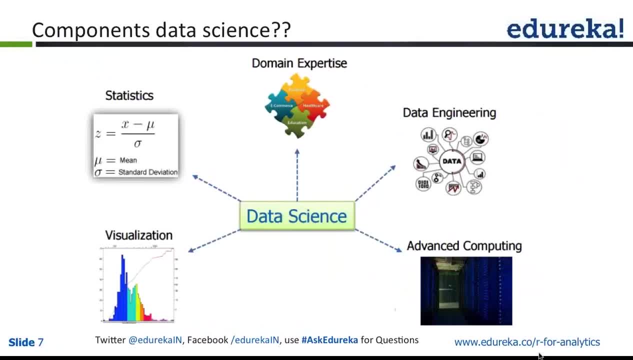 in statistics when you work on something which grows beyond realm of two-dimensional or three-dimension. that is where you need something like more advanced visualization that you can do in, and there are some libraries like d3. and finally, which is again a very important part, is called the. 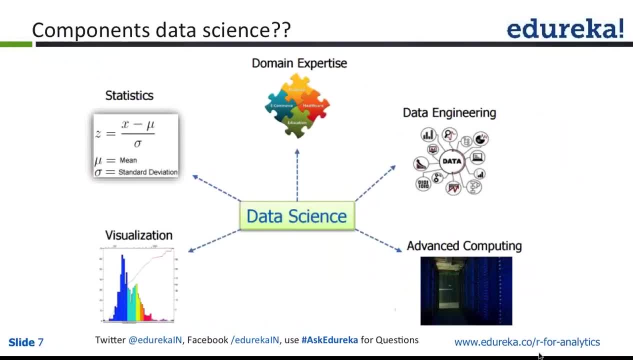 domain expertise, so you need to know the domain. for example, I'm a data scientist and I work majorly with the life sciences data, so I'm also an epidemiologist. so I have to deal with, you know, columns, with data set, with, you know, with more than 10 000 columns or 20 000 columns. 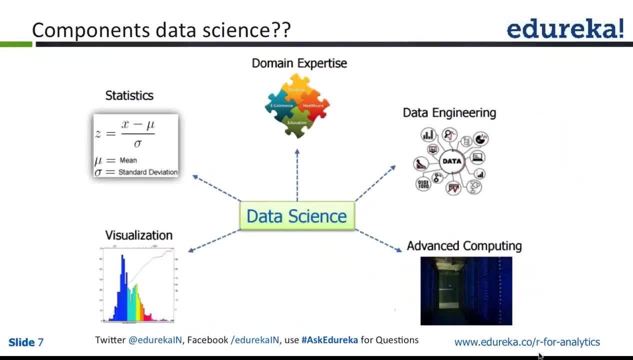 and that becomes really difficult for me, because running a analytical model with 20 000 columns is virtually impossible, so I need to have some domain experience to figure out what could be more useful in this entire data set. right, let's move ahead. so components of data science again. 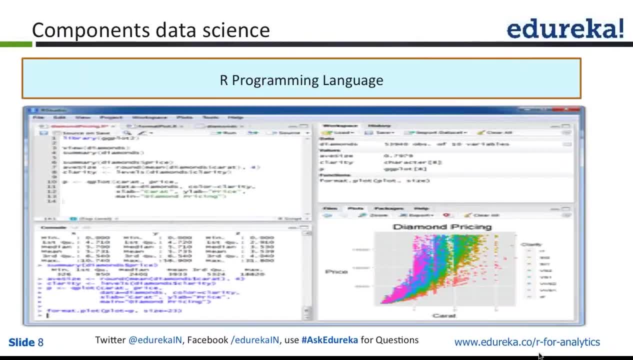 so our programming language. what possibly could R do here? R is a programming language. well, the answer is yes. is it similar to java? the answer is again a yes, because it is OOPS. it could be used as OOPS language, but is it mean for the same purpose as java? the answer is a big no. so we don't build. 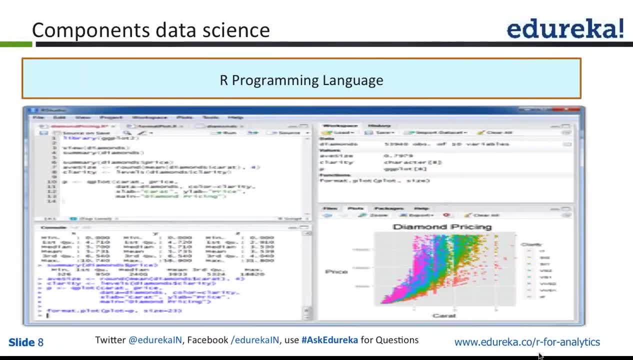 uh, we don't build any of the of these scripts or our programs in R just to serve a purpose of an application development. rather, most of the stuff that we do here is for a statistical modeling, so R is also called as the statistical modeling language. then this, this small picture that you see, is of an R studio screen where you've got where you can. 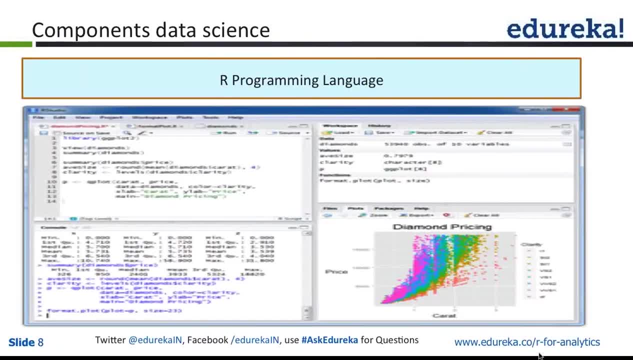 write a script and execute them in a console, which is the bottom left of this image. on the right bottom you see a plot. so, basically, R allows us to run all these kind of plots. they look really difficult at times and they difficult in the sense they they are hard to comprehend, but they are. 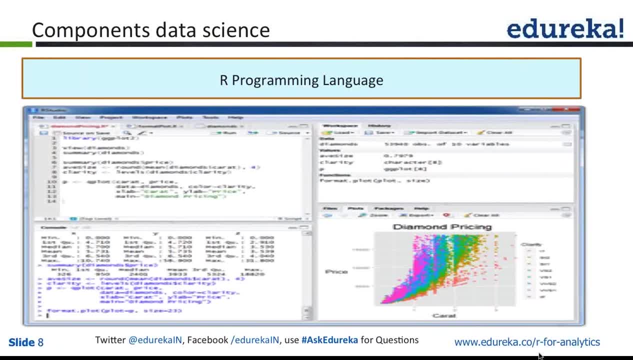 really meaningful and all these plots can be pretty easily generated and they are very difficult to understand. but they are really meaningful and all these plots can be pretty easily generated. and all these plots can be pretty easily generated, generated. and R? well, it assigns demand supply gap. now, why the hell? 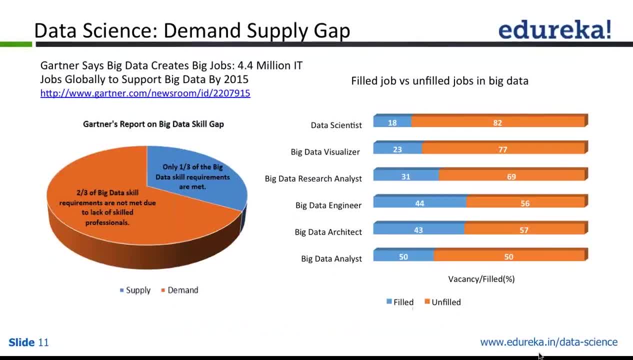 should we think of switching our careers to data science and big data and all that stuff? well, i don't know if you've been to Gardner. i've been to Gardner like thrice, specifically for the bi and for big data, and data science is one skill that Gardner consistently advocates on. 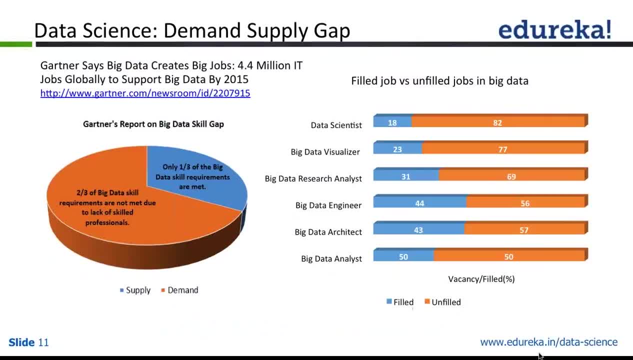 and that's because industries are now figuring out that they've got data and they can do something really important with the data. so what exactly is that? is that a data scientist would do? where a data scientist can channelize your not usable data or unused data into? 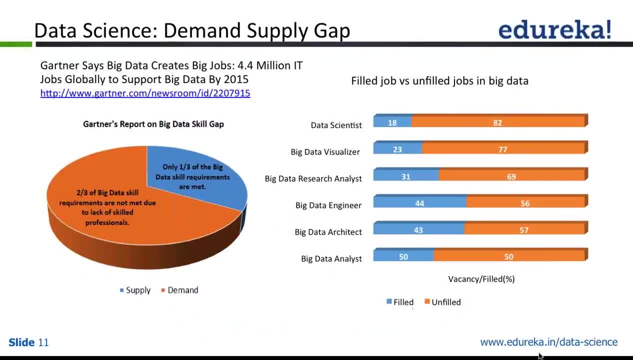 something is really meaningful. so think of a scenario where you got data about your parking in particular mall. let's say you got data about which car was parked at what time slot and when and what was the car type and on all that information about the car, can that be used by a store that is built in that? 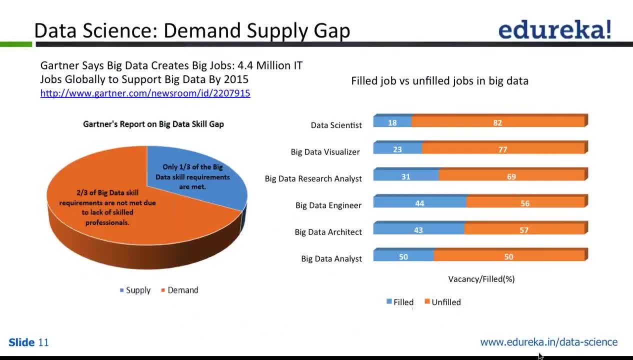 same on a retail store- a retail outlet of that's, a Walmart- to predict what is the amount of ice cream breaks I need to store in my refrigerators, based on the information that I get from the parking lot. but of course they had that information. but with data science now they can find correlations. 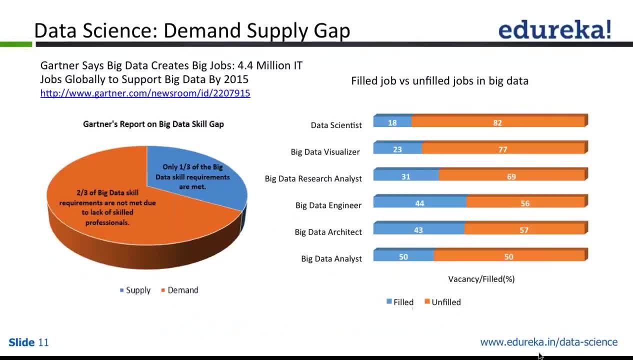 and that can help them understand or come out with a number that will ensure that they don't fall short of these ice cream picks. well, in the current scenario, the industry currently is in a big need of data scientists, which could be, in fact, and all these versions that you see: data, big data visualizer, big data research. 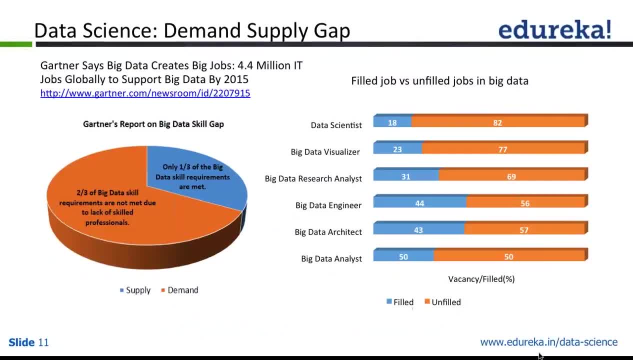 analyst big data engineers, architect and analyst- whatever all these guys are actually one or the other form of data science that can help them understand something about the food market as a data scientist and a data, and is supposed to be actually a combination of all of them. so you need to know. how do you need? 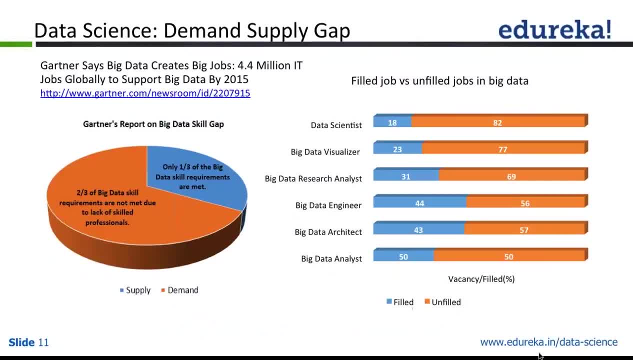 to know. you need to know big data. you need to know a NoSQL or a columnar database like MongoDB or edgebase, which is more columnar. then you also need to know the statistical part of it, which is, I think, the most difficult part: the algorithm's, the data preparation, that every, the data visualizations, all that a. 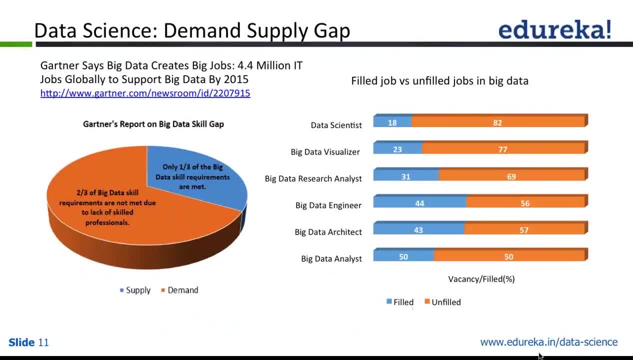 would constitute the work or the skill set of a data scientist And, as you see, currently only less than one third are other vacancies that have been filled and companies are ready to pay higher salaries just because this is a very rare skill. And this is not about learning yet another technology. 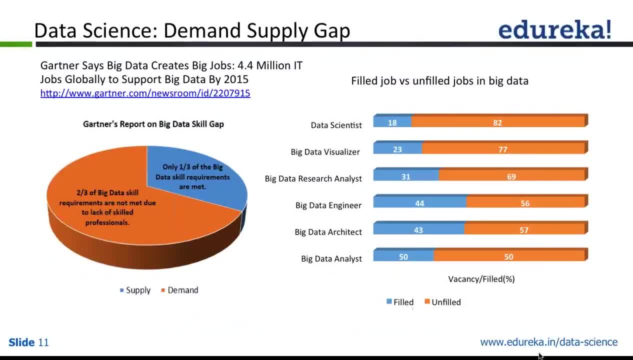 With data science. you need to master some of the math, you need to master some of the linear algebra, you need to master matrices. you need to master machine learning, you need to master programming. Then there is Hadoop, and then there is Spark, and so on. 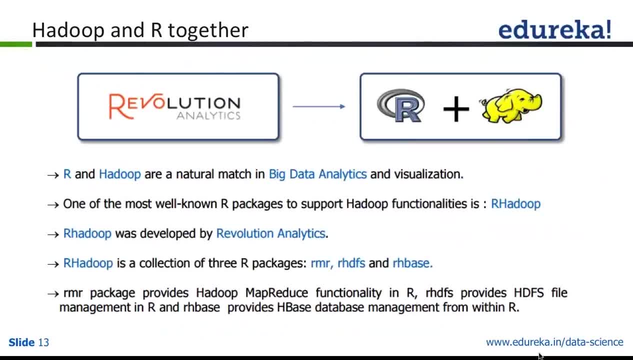 and so forth. So Hadoop and R together. So with R there's a problem of RAM. So R basically is in memory. That means it fits everything in the memory and then runs. So if the data set is not small enough, 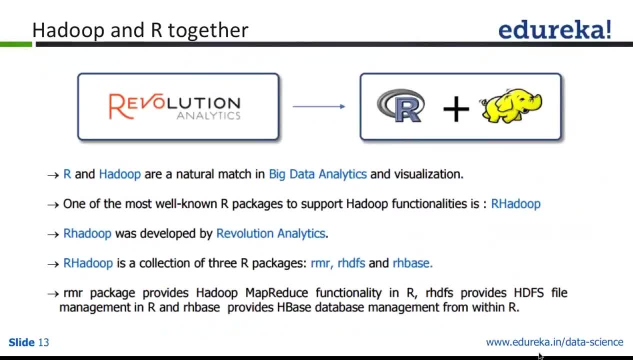 or it's really big that it cannot fit in your RAM, then you need something like an R and a Hadoop combination where you can run different folks or different threads of the same R processes on different machines. That is provided by a technology called as Revolution Analytics. 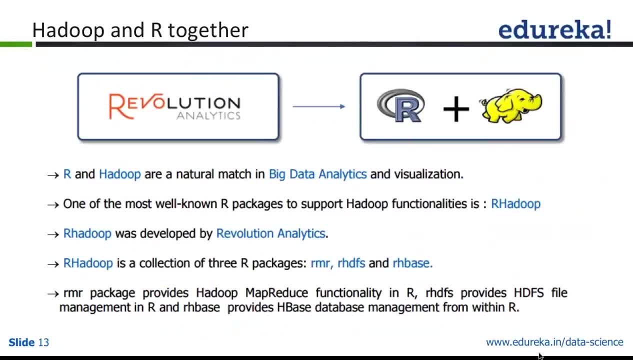 Revolution Analytics, by the way, was bought by Microsoft in the very starting of this year. Revolution Analytics has done nothing, but they've combined R and Hadoop using a package called RHadoop, which is a combination of RMR, RHGFS. and RHBase. So it's a combination of RMR, RHGFS and RHBase. So it's a combination of RMR, RHGFS and RHBase. So it's a combination of RMR, RHGFS and RHBase. 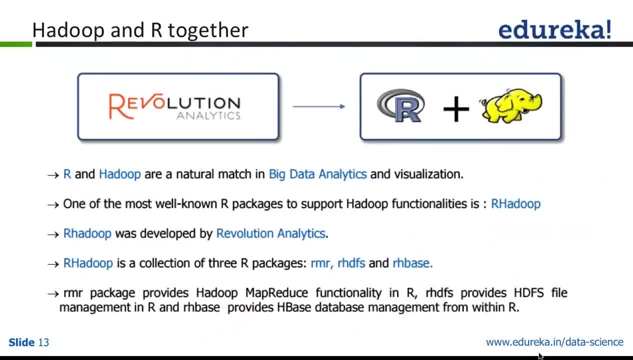 RHBase is something we need not to worry about right now, but RMR and RHGFS are the ones that allows us to read from HDFS, which is the Hadoop distributed file system, and run our program in parallel on all the machines. 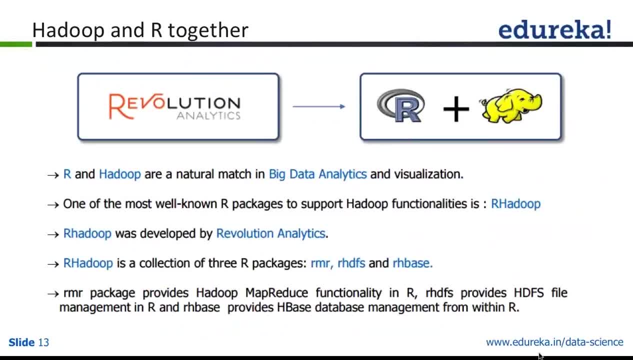 Obviously there are limitations to it because the algorithms like neural network or algorithm like regression, linear regression, that can't be done, That can't be made to run in parallel. So think of a Fibonacci series, So that starts with one, then one again and then two. 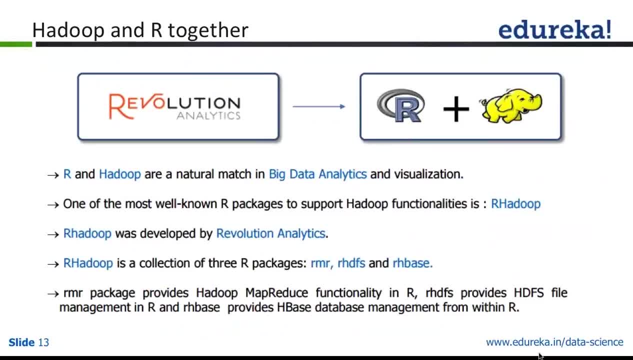 then three, then five, then eight and then 13,, and so on. So basically, it sums up the last two numbers and comes up with a new one, And then it sums up the new one and the second last one and then comes up with a new one. 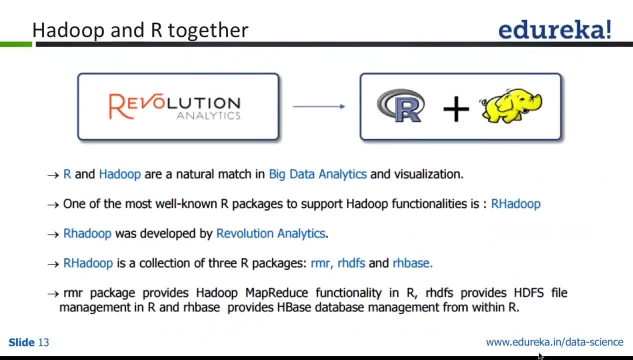 So basically we don't have the option of running it into parallel because the final step, or the output step, is based on the output step. So that's one big challenge with parallelization. So not everything can be parallelized, but there are certain algorithms that 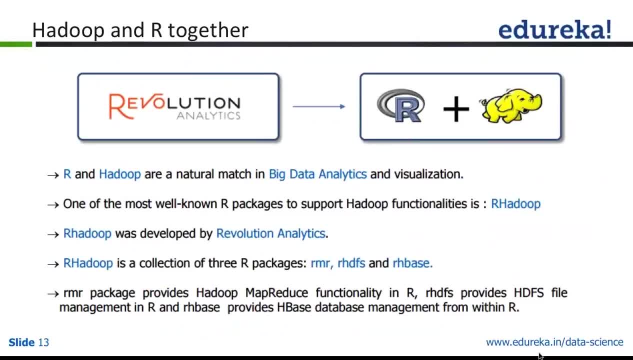 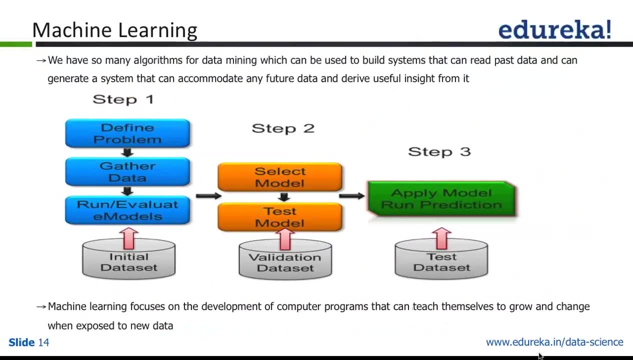 can be made to run parallel like support vector machines and random forest, So we can use them in this concept called RHadoop and thus minimize the execution time. So let's move on to machine learning. In machine learning, we actually don't go beyond the data lifecycle that you've seen. 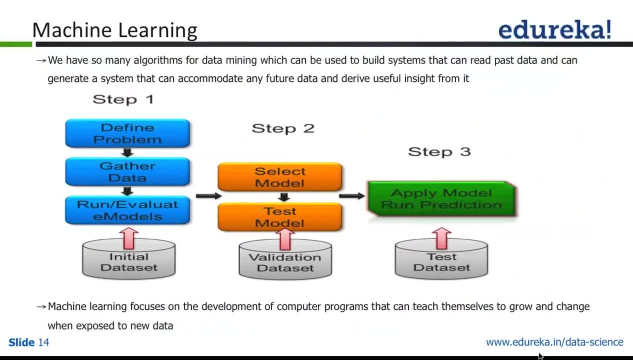 The only difference is that we start is with a different data set. So, basically, we have our initial data set on which we run and train our models. So this is called a training data set. So, whatever is your training data set, the algorithm will understand it. 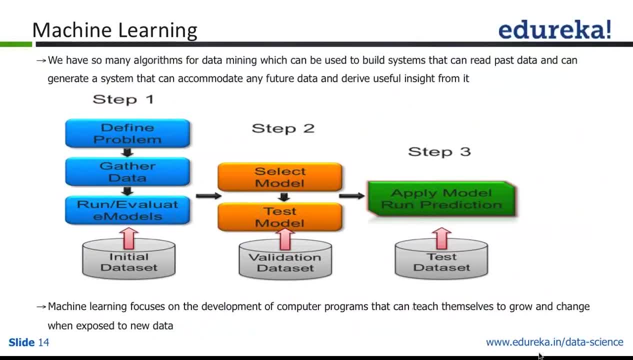 if you provide wrong data, it'll give you wrong answers. so think of it in this way: that you have a image of a duck and you tell the in guard, the computer, there are the algorithm, that it's a dog, so the, the algorithm will figure out this. these are: 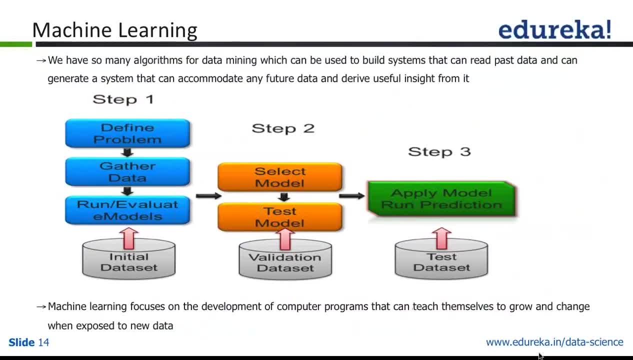 the particular features of this image, which is now framed as dog. so next time when you show it the algorithm, the image of a duck, it will call it a dog. okay, so garbage goes in. then garbage will go, we'll come out. okay, so that's called is. 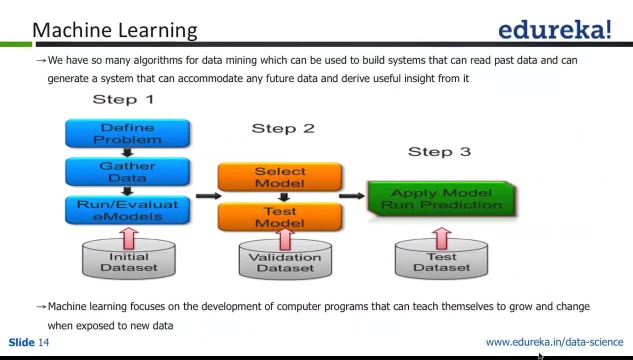 the training data set. so we run our, run our problems or run our algorithms rather on the training data set. now we have got a validation data set for which we know the answers again, but we ask the model to predict the values for us and based on that we get our predictions accuracy. 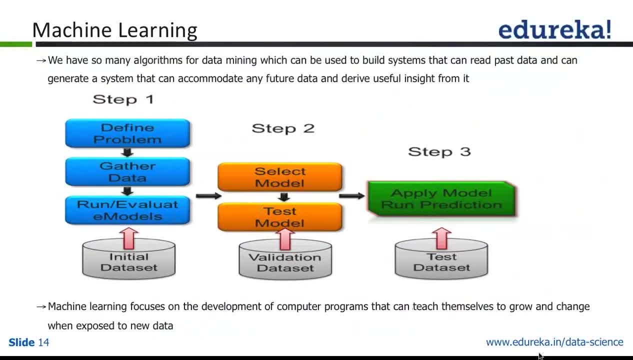 now what we do, that we run it on another data set called as a test data set or a primo data set. so the purpose of this data set is to keep it totally independent from the one from the developer who actually created those legal terms and that model, and run it in a production environment or a UAT. 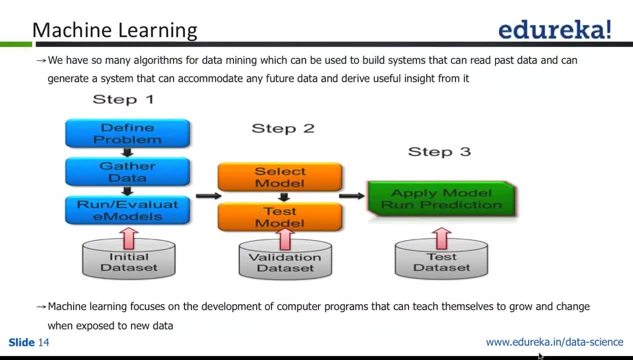 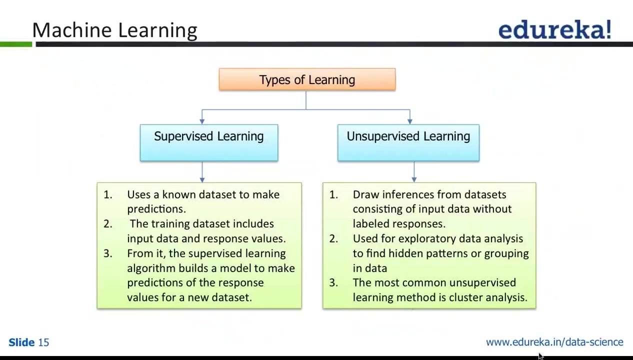 environment where the developer does not have access to any of the test scenarios. so machine learning focuses on the development of computer programs that can teach themselves to grow and change when exposed to new data. machine learning basically has two components: what is supervised learning, and the other is unsupervised learning. so what is supervised learning? I mean, I don't want. 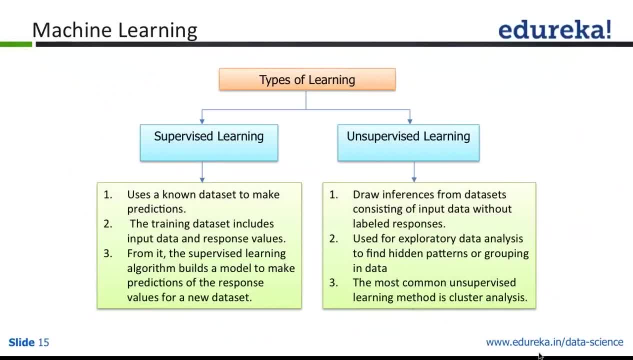 to actually go through this paragraph, but think of a case where you're as the problem is, you have to figure out whether a particular bank account will turn into a NPA or not. okay, that's the problem. so first you need a data set that tells you that these are 10 000 records and all of them were NPAs, and these were the next 10. 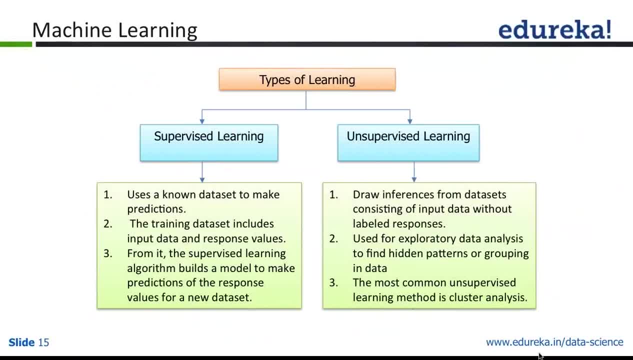 000 records and these were not NPAs. so the algorithm then figures out, based on the label- which is NPA or not NPA, that this kind of a, this kind of a feature, when used in this particular fashion, converts into a NPA and vice versa. but let's say you don't know the, the actual, the actual. 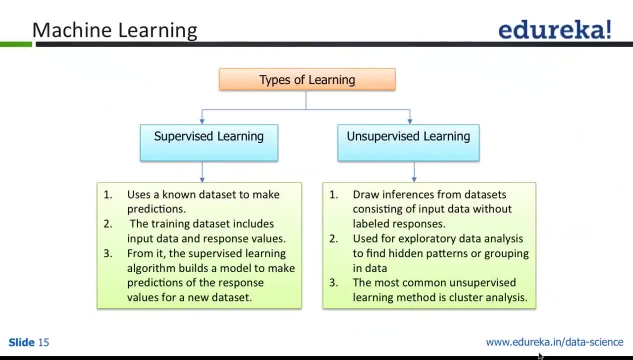 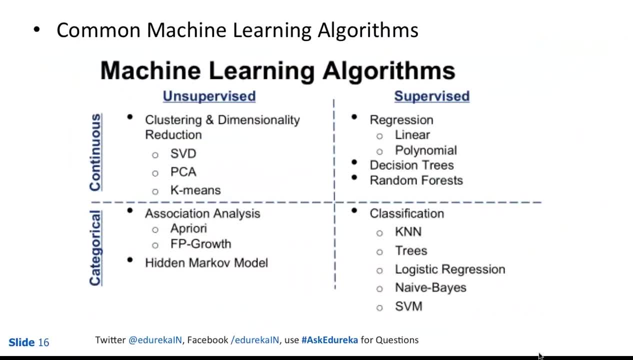 labels, but that's when you don't have the Y and that's a form of clustering. so, majorly, what we do in unsupervised learning is clustering or dimensionality reduction. we'll see it once we get into the lab. well, the common machine learning algorithms. 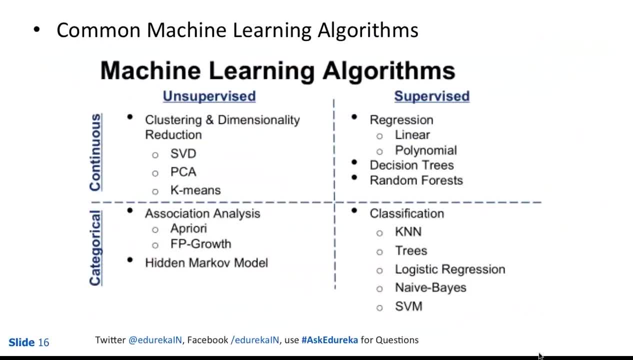 we've got two, two categories, when I supervise and unsupervised, that's what you're learning. then there is one called as regression, then there is one called as classification, then on, there's one particular step is called as clustering and dimensionality reduction, and the final is called 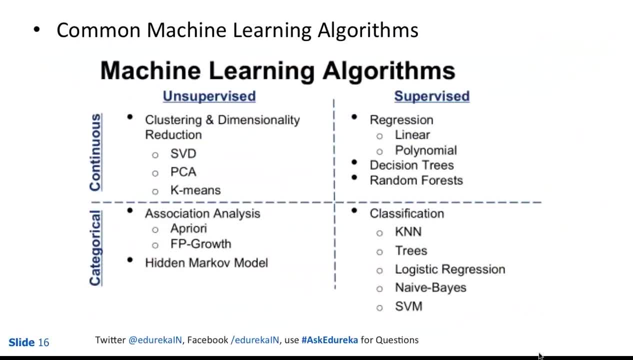 this and the final days. there's some more categorical. categorical unsupervised learning algorithms which are called as association analysis, basically figuring out if X is bought, then what are the chances of buying Y. so basically, in supervised learning we do regression and classification. so regression is figuring out what 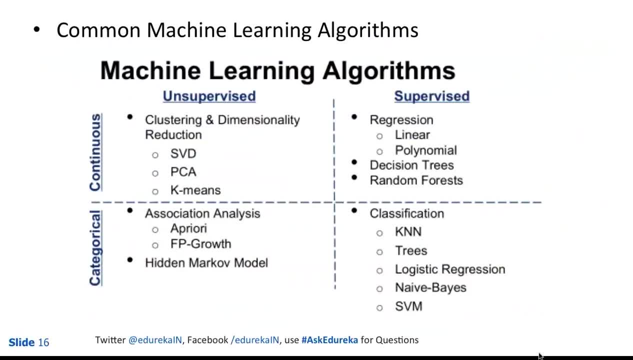 is the numerical value of a problem. so let's say there's a prediction analysis and you figure out what is the salary of a person, and then you figure out what is the salary of a person and then you to the 맞아, mean OK, okay, so what's? 3 is the total number of units. so this you have to look at the. 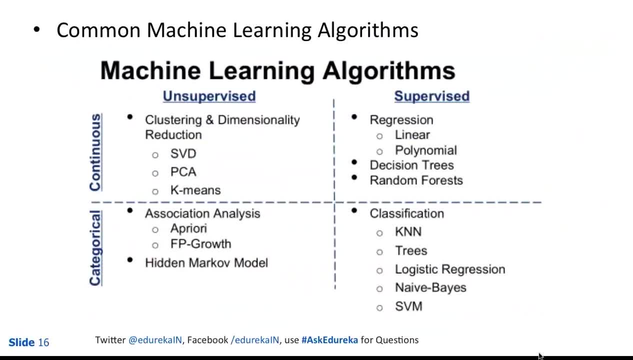 linear at that you to come up with. it's not high or low, it's not 1 or 0, so that's not classifying into anything. so, basically, when you predict a numerical value, it becomes a regression problem. of course, the way to approach a regression problem is: 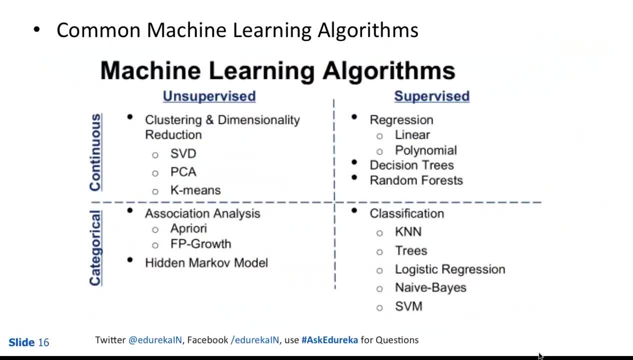 different a way to is different then way to approach a classification problem. now, of course, a see that then decision trees, a random forest. well, these are state-of-the-art algorithms. classification is when you want to classify a particular record into categories NPA, not NPA is a classification algorithm. accept the. 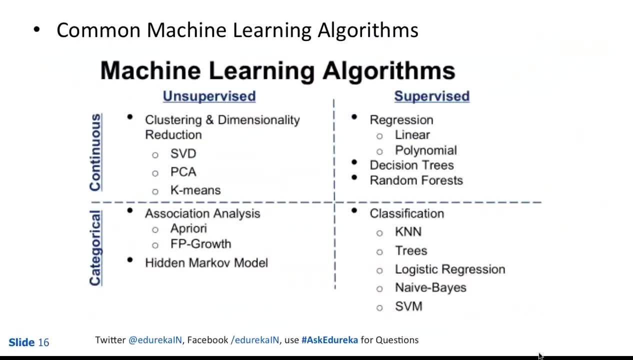 offer, not accept the offer. as a classification algorithm- good, bad, high, low. all these are examples of classification algorithms where you want to categorize a particular record, a particular document, a particular entity into one type or the other. then in the unsupervised, we've got clustering and 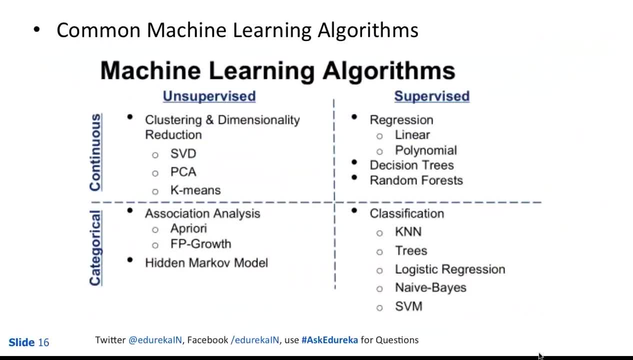 dimensionality reduction. so clustering is basically figuring out the clusters within the data set. so let's say you develop a guard them, develop a way to figure out how many kind what are the salary standards of a particular country? so let's say you want to divide the entire population to high or low, but you 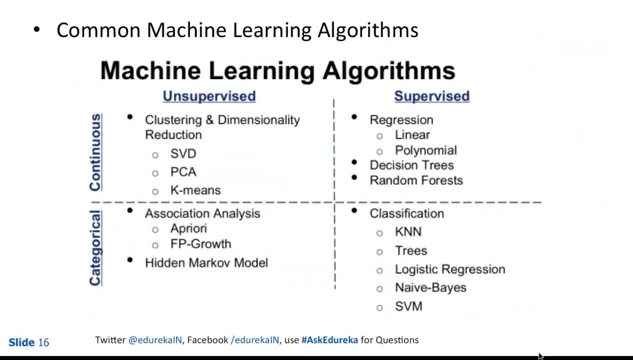 don't know where the particular salary is high or low. so what you do is you divide the entire population into two clusters, so one cluster is for the high income and the second cluster is for the low income. and finally, we come to association analysis and the hidden Markov models. well, these algorithms based on the 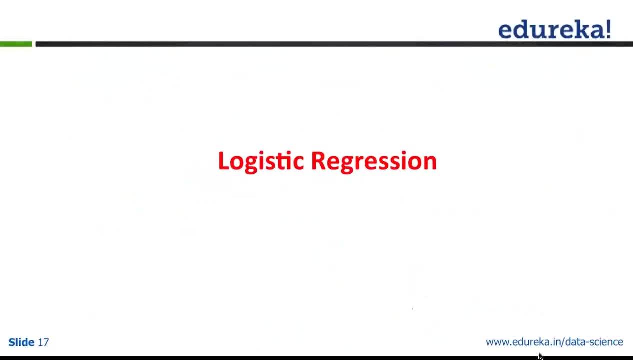 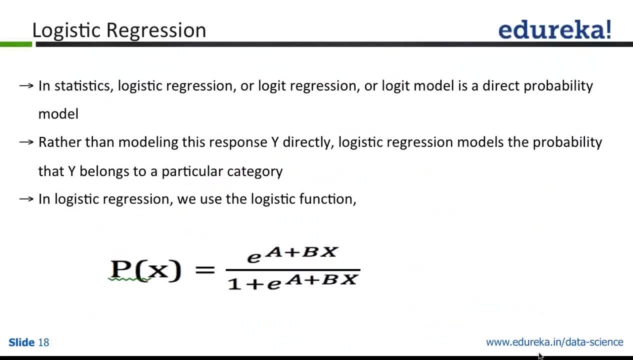 market basket analysis and you know, if one, then two kind of a concepts. okay, so now we'll come to the logistic analysis. so we'll come to the logistic analysis and we'll come to the logistic regression. so in statistics, logistic regression or logger regression, or logger model, is a direct probability. 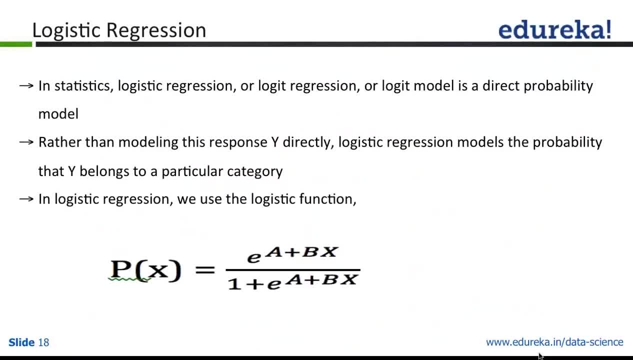 model. so I believe that all of you understand what is linear regression. in case you don't, so let me tell you that a linear regression is the one which has this: one y equals two a plus b x. so y equals three plus b. x is the standard equation for linear. 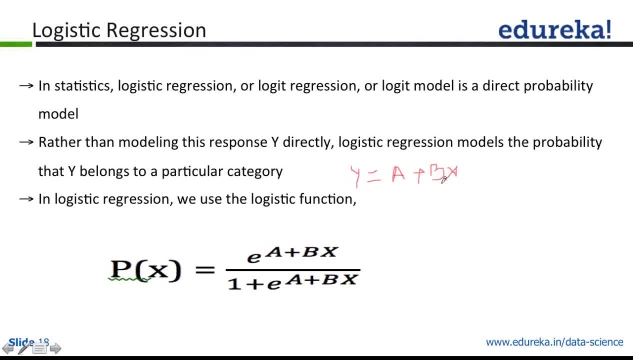 regression classifier, sorry, linear regression model. so what is x? x is your independent variable and y is your dependent variable. so X could be a value, it could be a variable, could be a matrix or a vector. what is B? B is the coefficient, so y equals three a plus b, x. 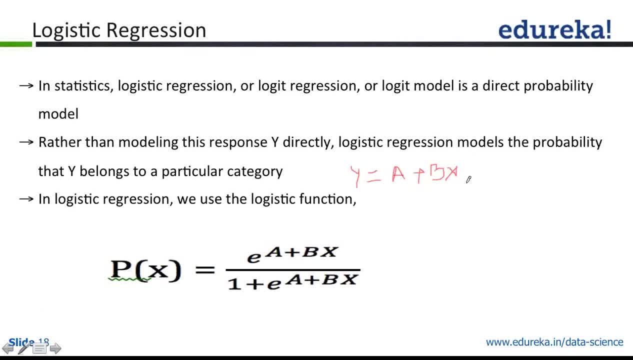 is actually the equation of a straight line in a 2d geometry. so a is the intercept and B is the slope of that line. so basically we determine slopes using concept problems, these squares. and that is how we figure out the optimum value of y, by fitting a curve, a straight line, in a linear regression in logistic. 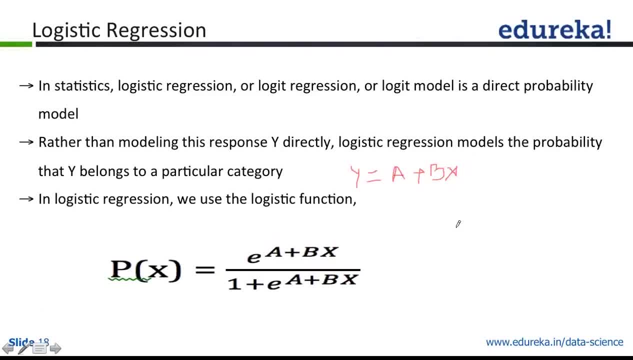 regression. we use the same concept but we apply a sigmoid function. a function whose value is f of X is equals to- i'm sorry, i'm writing through my mousepad and on my Mac it's not that great- one upon one plus e power, minus x. so if you now, x in this case is our y, so f of y is equals to 1 upon 1 plus e power, minus y. 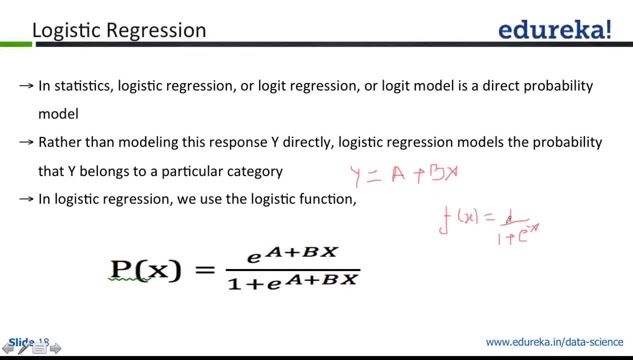 and that is nothing. but y is equals to a plus bx, so we'll get 1 upon 1 plus e power minus of a plus bx that will come down. and finally we'll get p of x, which we define as the probability of a particular event, as e upon e power a plus bx upon 1 plus e power a plus bx. 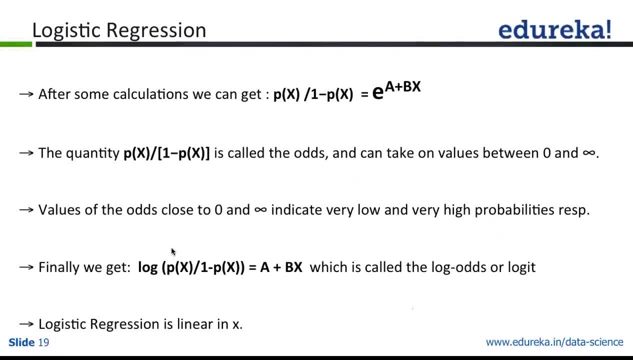 so after some calculation you get px upon 1 minus px is e power a plus bx. so the quantity px upon 1 minus px is called the odds of an event and k and can take on values between 0 and infinity. that's because it's raised to the power e plus e upon e, power a plus bx. well, values of the odds. 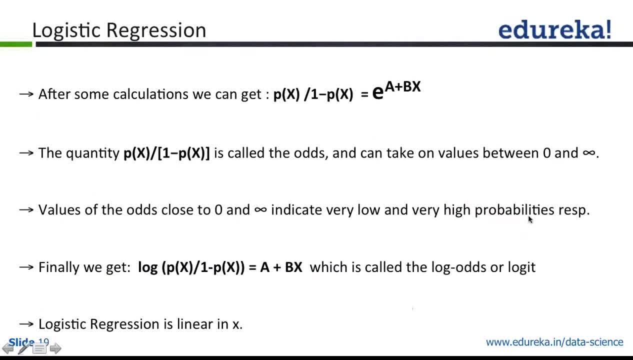 close to 0 and infinity indicate very low and very high probabilities respectively for an event. so we'll get px upon. 1 minus px is e, power, a plus bx and k and can take on values between 0 and infinity. so let's say, if you get the value of odd as 9865, which is not a small number, 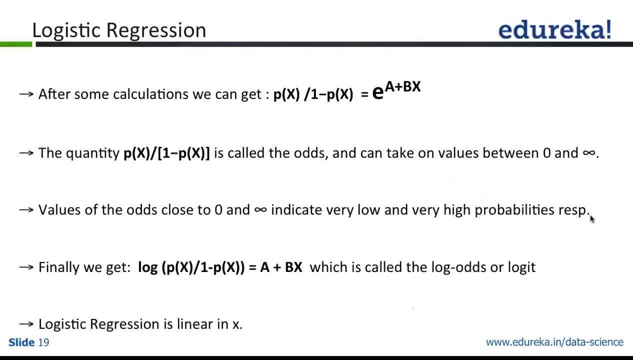 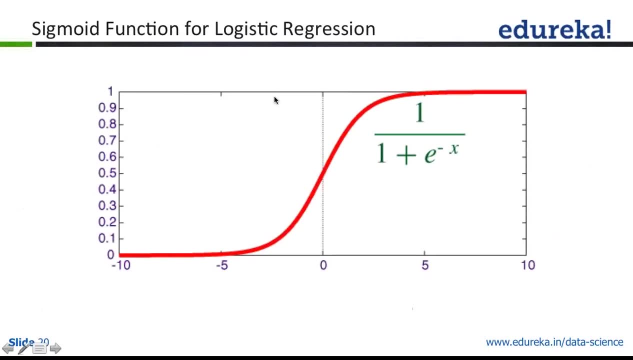 we'll say the value of the probability of that event is very high, whereas if we get the value which is like 0.84, then you'll say the value of of the probability of that event is very low. so when you solve this equation again you get: i'm sorry. 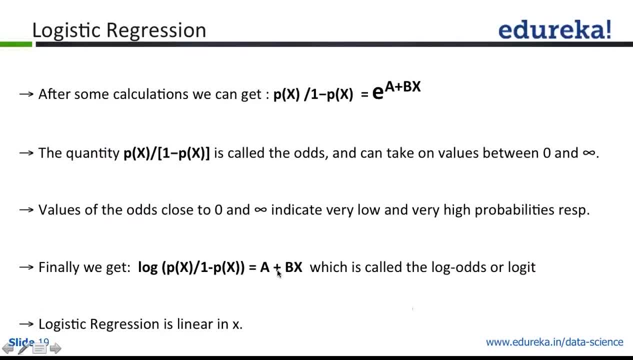 you get log of px upon. 1 minus px equals to a plus bx. so you see, a plus bx is the equation of our linear model and that is why this particular function is called as the logit function, or the logit function, or the log odds, and that's why we see that logistic regression is linear, with respect. 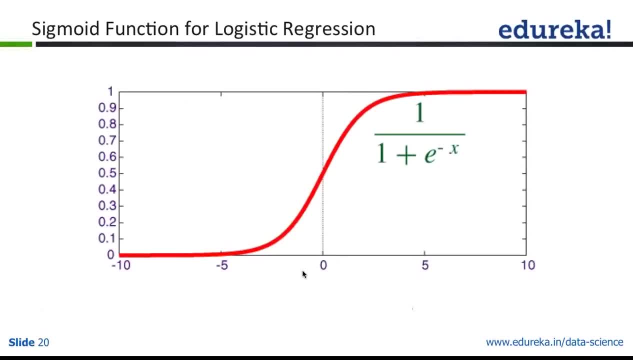 to x. well, this is the logistic regression, uh, sigmoid function. it has some very interesting features, you see. so it is: the value is closed between 1 and 0 and it crosses x equals to 0 at y equals to 0.5. so, when x equals to 0, y equals to 0.5. 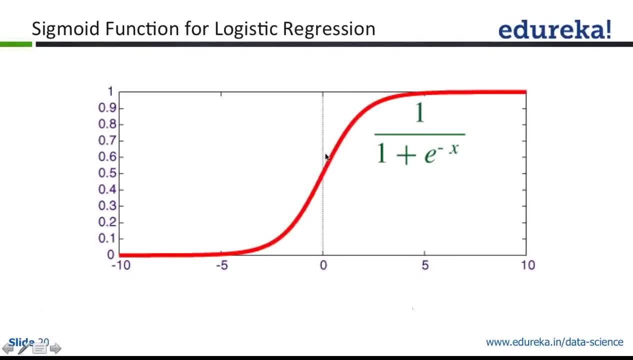 so that means if we are looking to figure out whether a particular count will be an np or not, then we just need to see whether the value of the sigmoid function that we are getting for it is it greater than 0.5 or not. it was greater than 0.5, then we say that that for all those value of 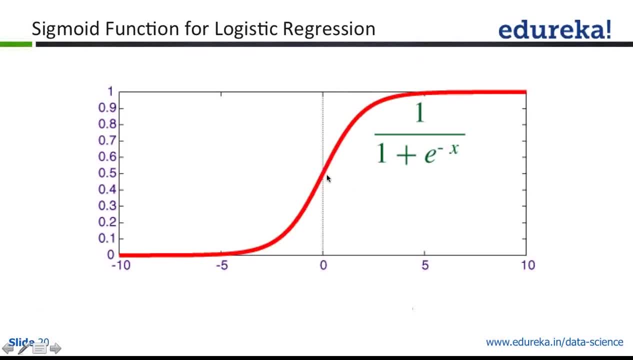 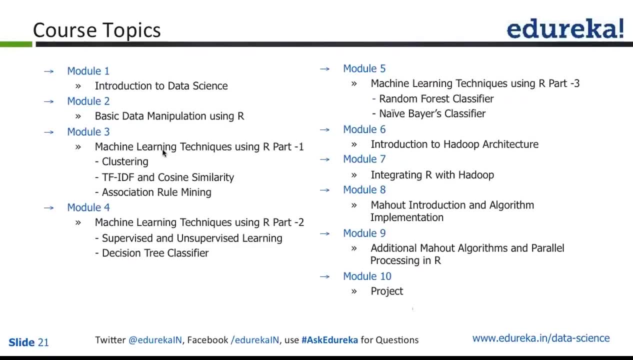 x, the category is blah, blah, blah, and for the rest of them the category is blah, blah, blah, okay, okay, so we do run our machine learning course in Edureka, and well, these are the modules of that particular course. we do basic data manipulation through R. we do a lot of stuff in text analytics. we do. 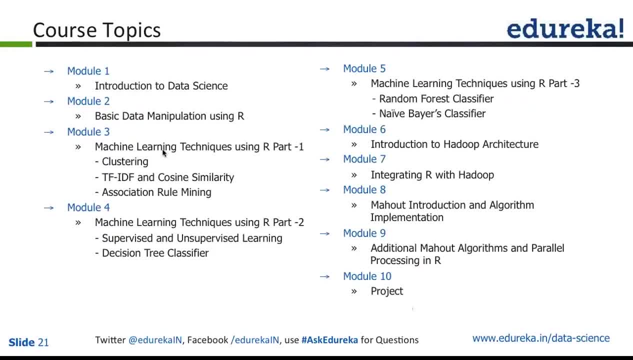 we go through the state-of-the-art machine learning algorithms, right from random forest to naive Bay's. finally we go on to integrating Hadoop and R. we also learn certain set of stuffs on my house and machine learning in Hadoop, and finally parallel processing in R, and then we've got a project. well, that's. 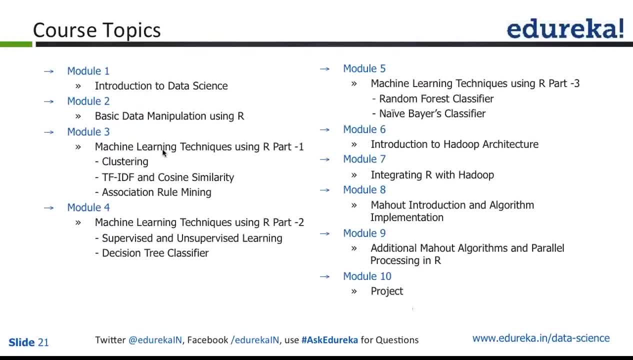 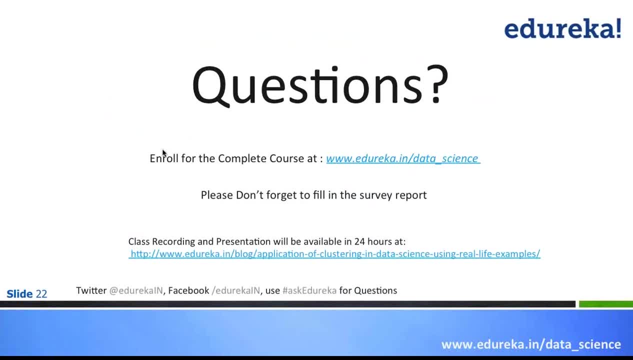 that's exactly what we've been doing so far as part of the data science course in Edureka. well, that's the end of the slides, but that's not the end of the session. now we're going to go into the hands-on exercise for logistic regression. 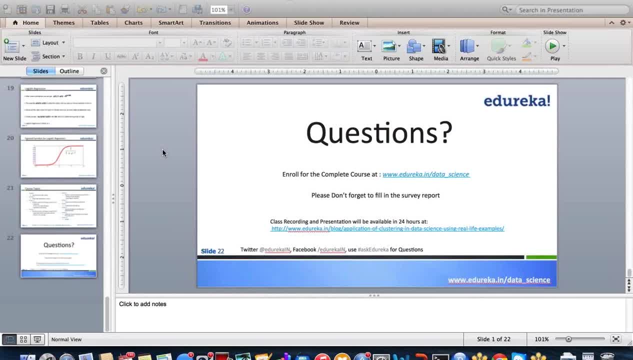 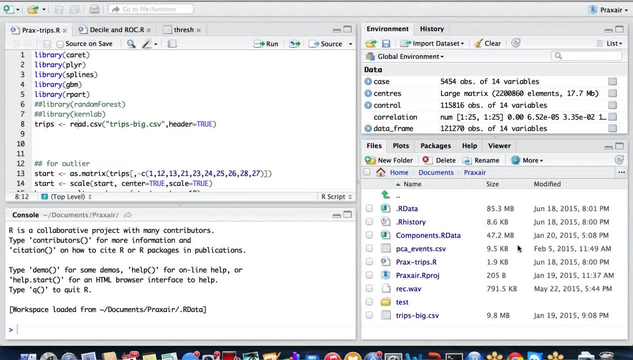 so I'm going to open up my our session. I hope you all can see my ask our session. let me see God forgot a question. well, it seems like some of you've got questions, so let me see how many questions you've got. okay, okay, so I see some of you guys. 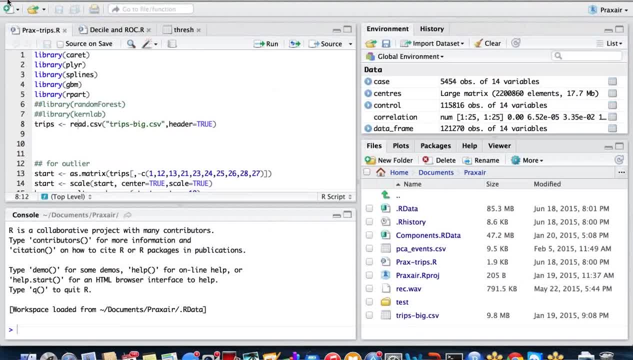 have the problem you are with the wise, but it sees that it is. it seems that are some of you are able to hear me. ok, so we did the questions after the session. ok, so let's start with our ok now. the problem then will solve is regarding: 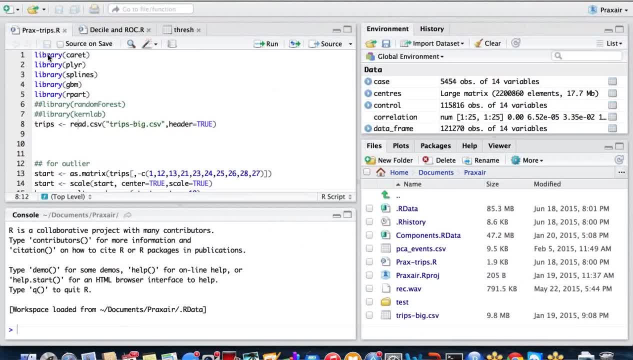 our organization wanted to figure out that. can we? can we predict a particular trip as risky or non risky? risky means whether there are chances that that the trip will have an accident. okay, so this is about a company jet that transports helium in big containers and any blast nearby or even a collision with that, with that trunk on. 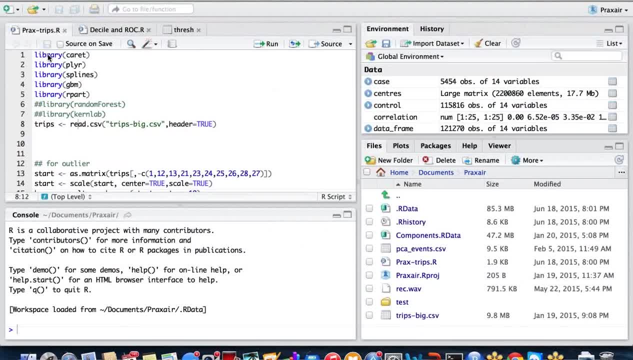 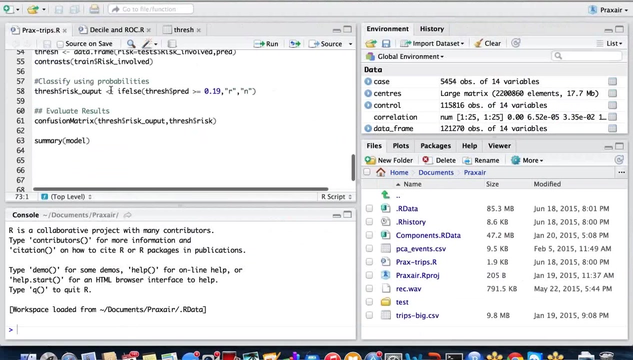 that container can cause even bigger explosion, explosion that can go up to 100 meters, which is huge. so they want to ensure and they want to be extra cautious about, about figuring out a possibility of an accident. okay, so we're going to use some libraries once this library is carried, so, oops, I'm gonna. so. 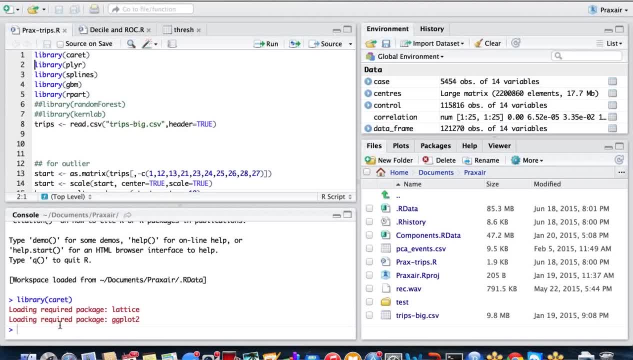 the moment I enter here I see the output on my console. so I have entered this carat library and I've entered in the carat library zone. I use plier. I don't need spines and our parts I can leave that. so I've got a trip data set. let me, let us. 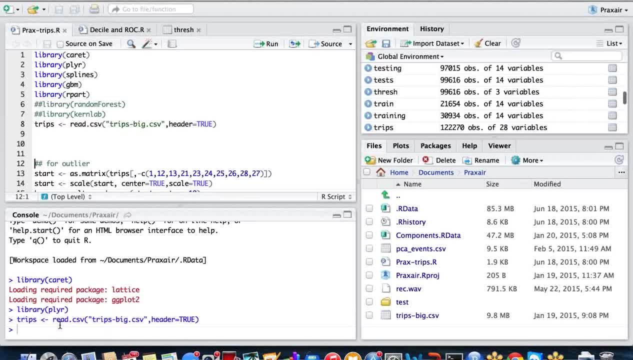 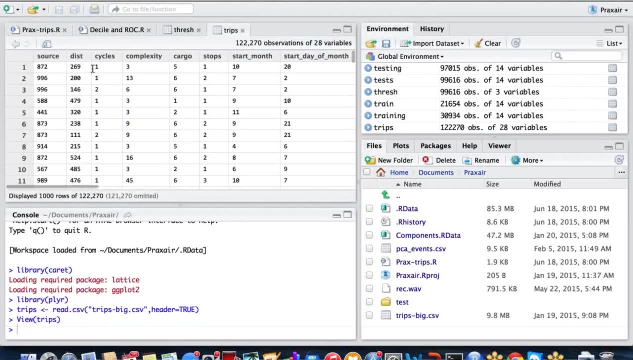 see what is this trip data set. so we are reading from a CSV that's on the machine. so let's see what is there in the trips data set. well, if this is the trip data set, source is the- is the one who is actually creating the schedule. distance is the distance of the. the trip is. 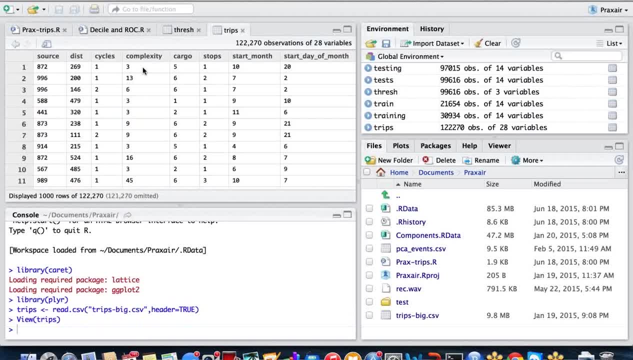 supposed to make cycles like: is it going to be a round cycle or is going to be a one-way cycle? complexity is based on the highways traveling on. then cargo: is it carrying a car going on? how many number of stops does it have in between? what is? 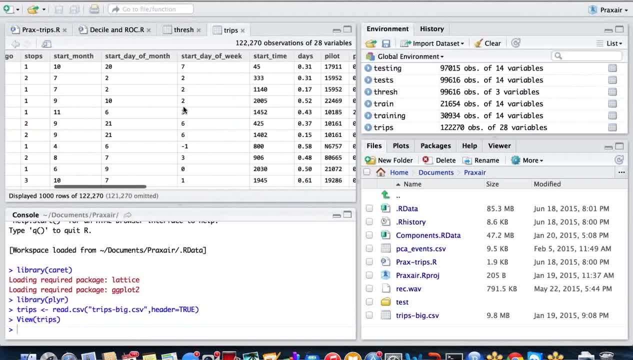 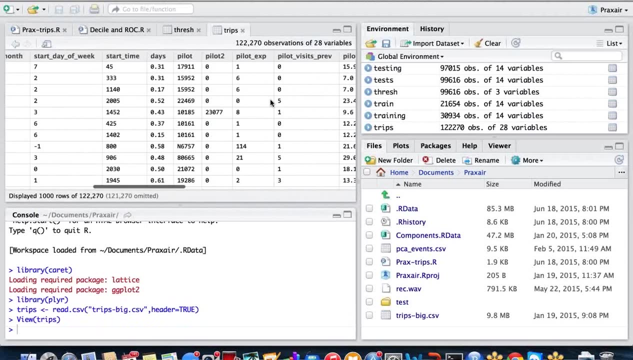 the start. what is the month in which it's starting? what is the day of the month? what is the day of the week? for example, if someone is working on a Saturday on the last week and the chances are high because the person is already tired walking throughout the week, start time is in seconds. then then 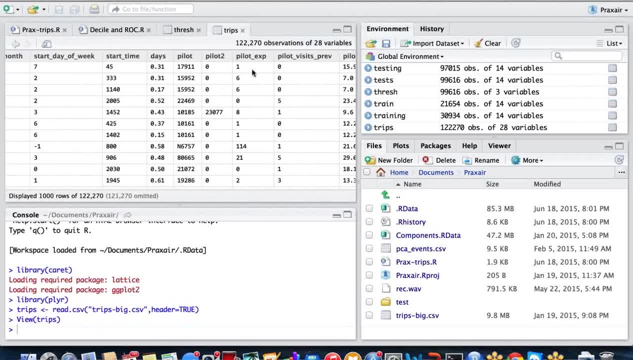 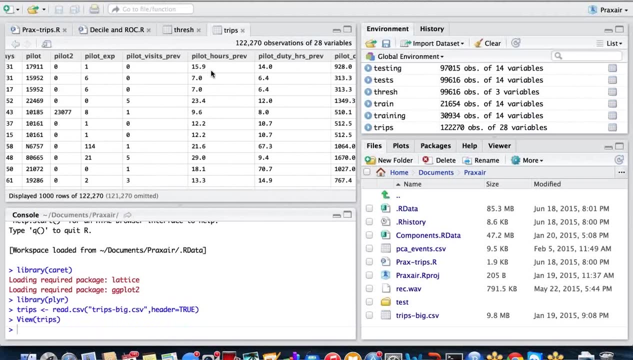 there's experience level in number of years, a number of months, so that's into pilot experience, pilot two. in case you go out, a pilot two, that means you've got another driver along with the main driver. then how many number of hours did the, the pilot or the driver drove in the last? 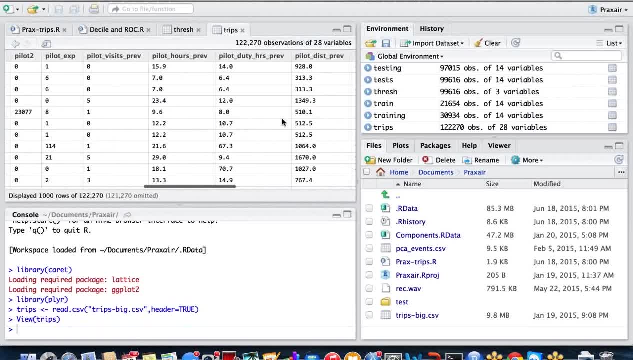 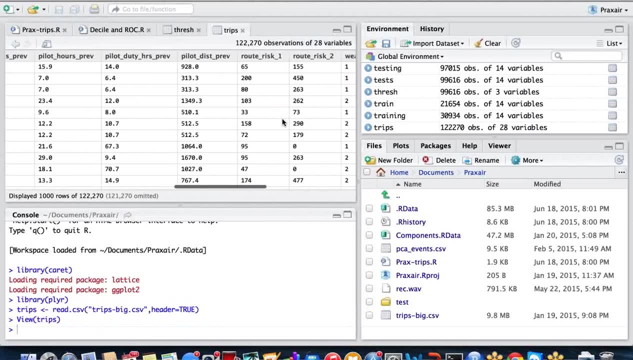 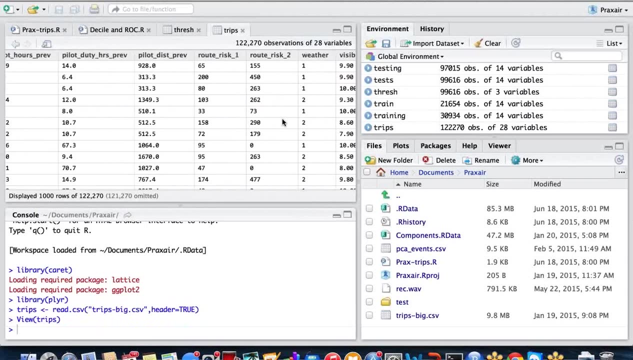 trip, okay, then pilot duty hours previously, then the distance, the, there the route risk underscore one and route risk and it's underscore two. so basically they've given a risk measure to every route and there let's say, if there are two routes to reach to a particular particular destination, then 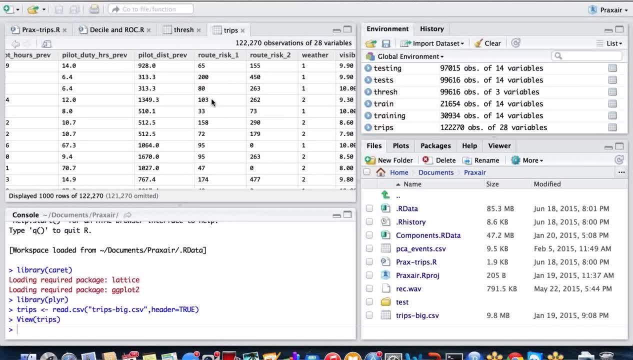 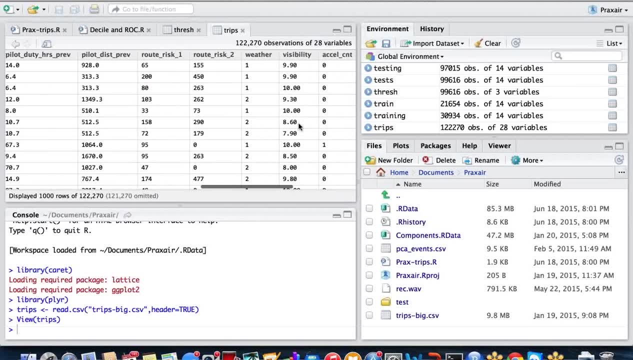 this could be. the route risk is the one route risk is the one for the first first route and the second one is for the second route. whether it's is it good or bad is like according to one and zero visibility is is taken to numerical factor. they have quantified it using a. 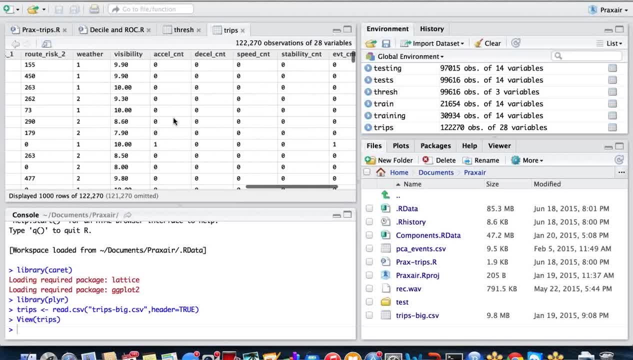 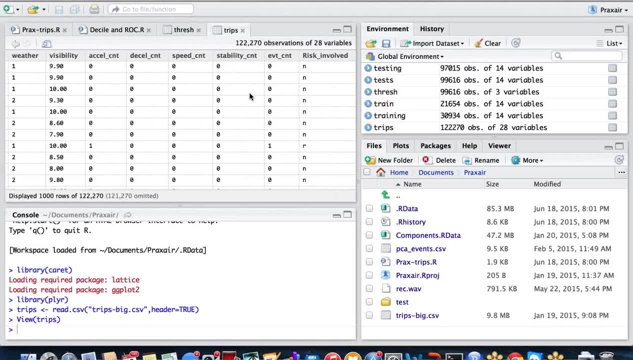 number, but is it a good or a bad visibility on that day? then we've got even like acceleration count, the acceleration count, speed count, stability count, even count. so if we have any of these value equal to one or more, then we define the trip as risky. clearly this is a supervised learning algorithm. okay, because we already have. 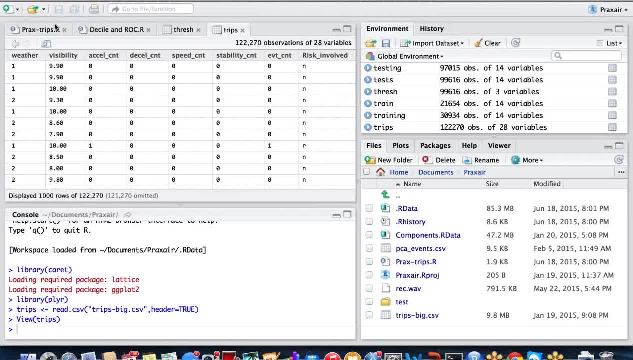 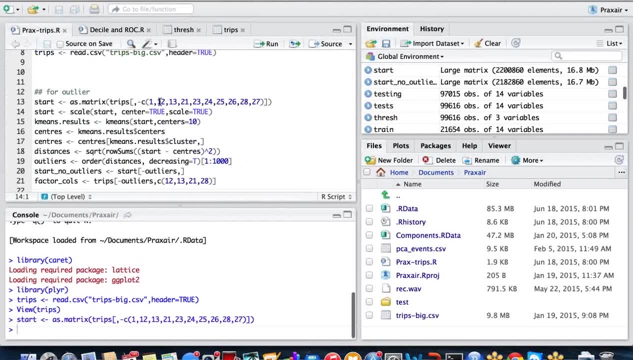 the risk involved, marked as yes or no. so let's go ahead. so, first of all, I create a matrix, start matrix. so I've just, so, I've just. I just chose the column that I need for my. for this prediction, I am now creating clusters using algorithm called 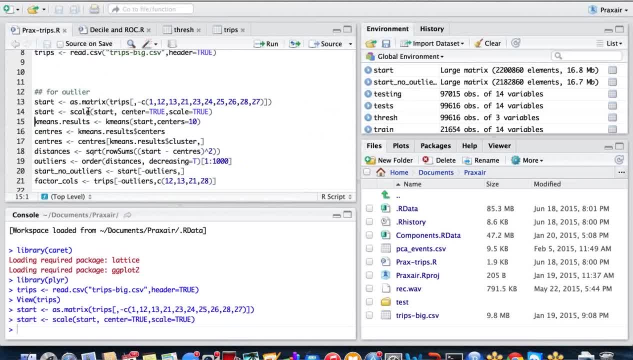 k-means cluster. right now I'm I'm going to call it k-means cluster. right now I'm going to call it k-means. take the struggled data set, but also a mean a. this way I've Centiro��이 내 dataset. quickly scaling the data set means. 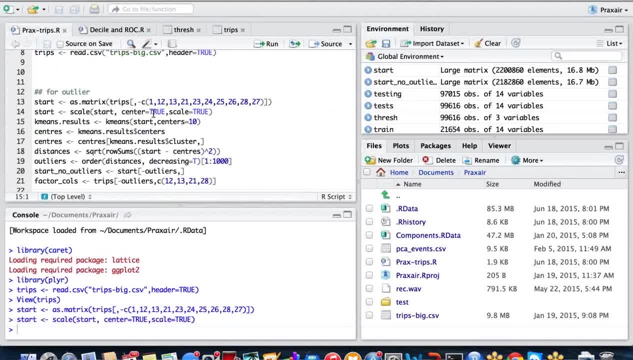 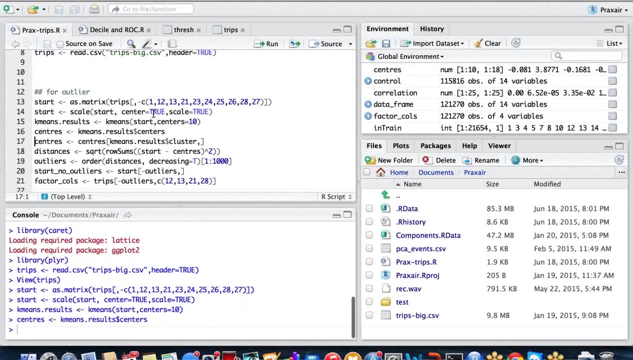 normalizing the dataset. by scaling the dataset means normalizing the dataset. so you did up besideанию divide by you divide by the standard deviation. thenício křmen khi zehn. scroll using the line called k means: with this you find the centers of those clusters. now you find the results of those centers into a column called. 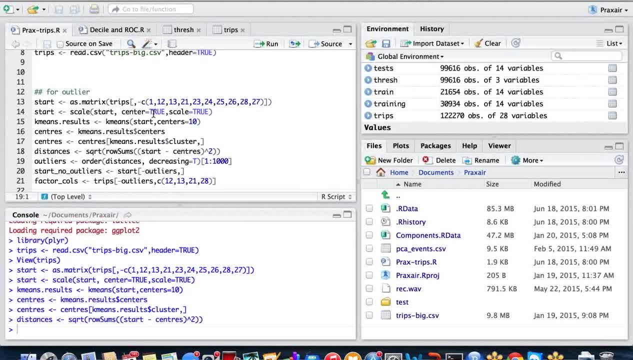 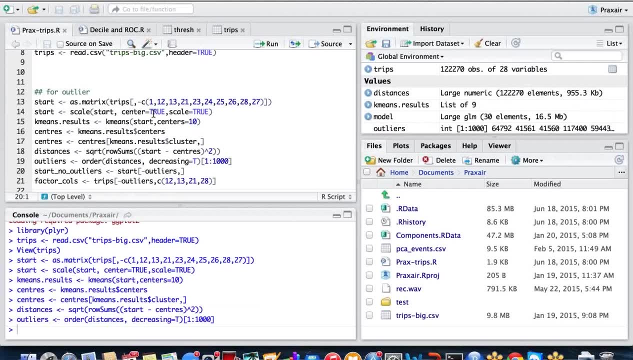 results and then you find the distance of each point from the center and then you find out which are the most distant points which we can point as outliers. so i've chosen one to one thousand which are the outliers guys. in case if you feel like this is not making much of a sense, it's fine. 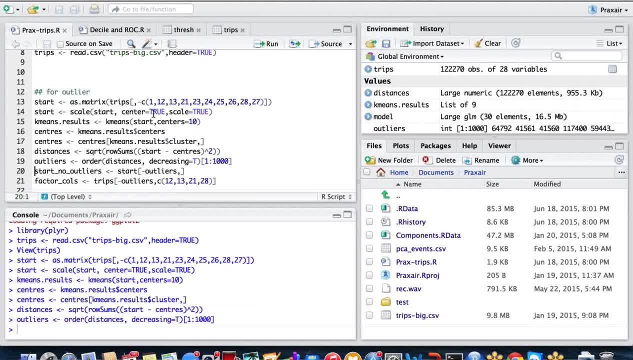 because if you're not from our background, if you're not worked on on any machine learning algorithm so far, it's going to look like french. but my idea is to show you how we run things and how practically, or how you know, uh, how hands-on are we with respect to our course? okay, 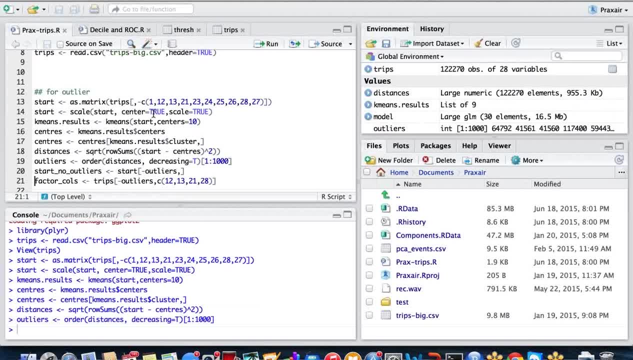 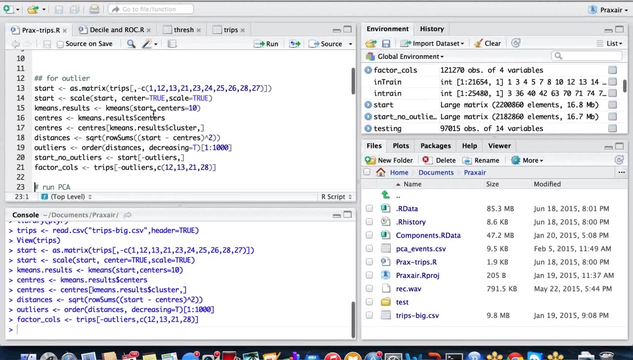 then we use, we convert the- uh, the trips, call the trips data set into factors. factors, nothing but any, any variable which has a value other than number. so let's say, uh, a gender, male, female, uh, the height, lower, high could be the variables which we can call as factors. so now i'm running something. 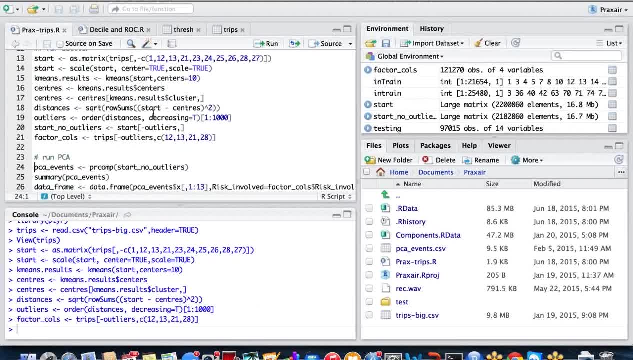 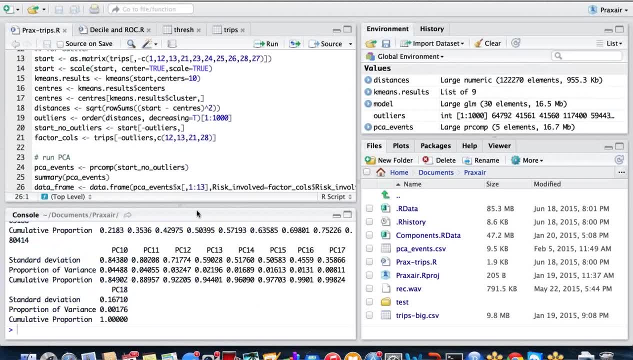 called as a principal component, analysis, which is reducing the number of variables. so so we've got, we've got 23 columns, but we can use only the first 13 to figure out those which which, which gives us accuracy of 0.94 to figure out further predictions. so that's the beauty. 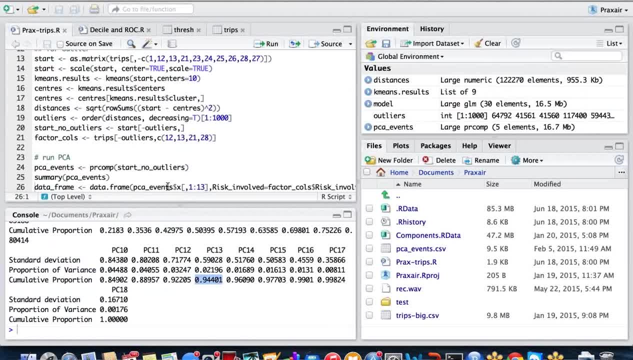 of. that's the beauty of principal component analysis. of course, we need not to go into the depths of it. see, i did say that we are running a supervised learning algorithm, but i've used two concepts, which are non-supervised or unsupervised, which is principal components and clustering. okay, 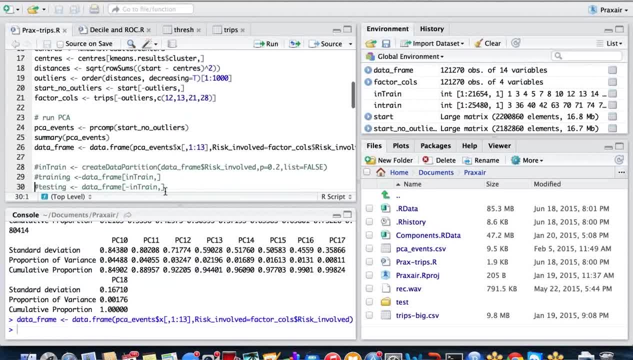 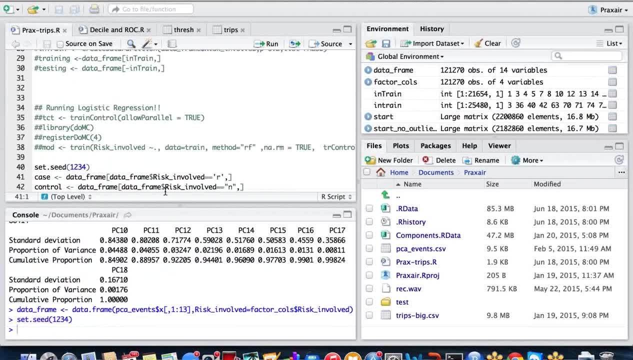 so i created a data frame with those principal components, principal components, and now i create. now i create something called as the case and the control data set. so the problem with accidents or problem with certain machine learning problems are that the act, the required events, are pretty less so think of, think of figuring out whether a particular 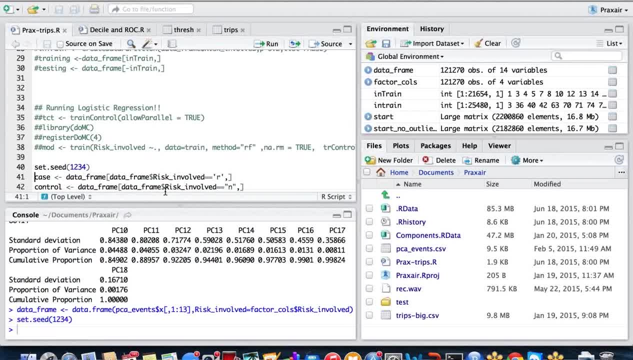 person will have a cancer, will have cancer or not. so we need data sets with people who have cancer and data set of people who did not have cancer. so cancer is- i mean cancer is pretty common nowadays, but think of it as a very rare disease and and, and, and you know, and think of it as, as like one in. 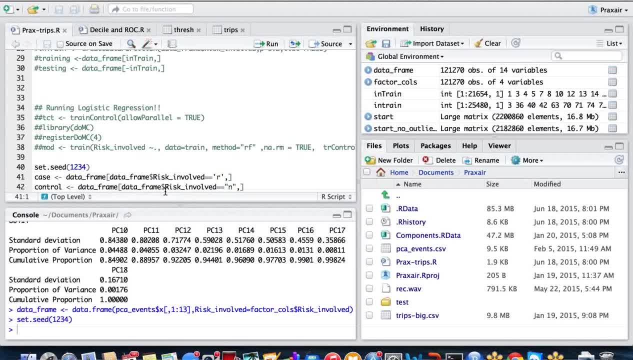 hundred kind of a disease. so basically what you've got you'll have 100 people and only one guy who have cancer. or let's say you think about uh the, uh, the click-through rate. so basically you are given, you're shown an ad. now i need to figure out the probability that, whether you click on this ad or not, 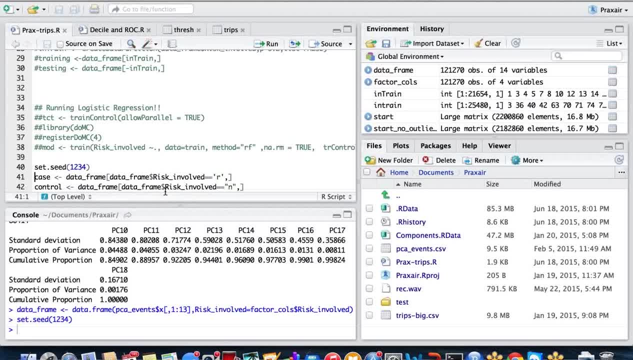 so to do that you need to first figure out the, the features of those guys who clicked on the ad. now the the ratio is one in one thousand. so in one thousand folks only one would click on the ad. so basically the number of actual cases are pretty less. so what we do is we do a sampling. 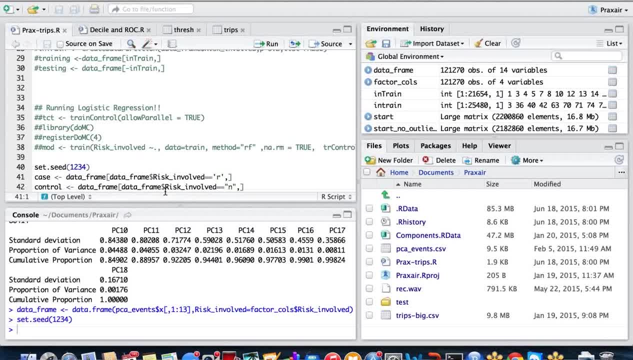 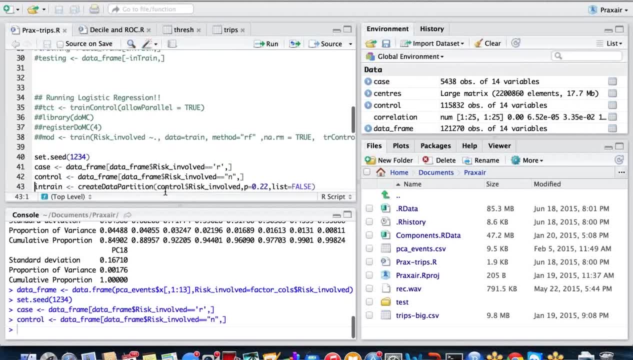 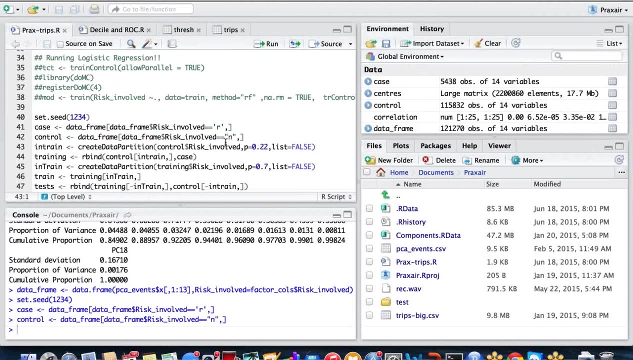 a strategy called as a. we run a sampling strategy called as a case control sampling strategy. so so we take all the data where we did find a risky data set and we take a part of the data where we find non risky data sets. okay, such that the ratio is not more than 1 is to 5. now we create 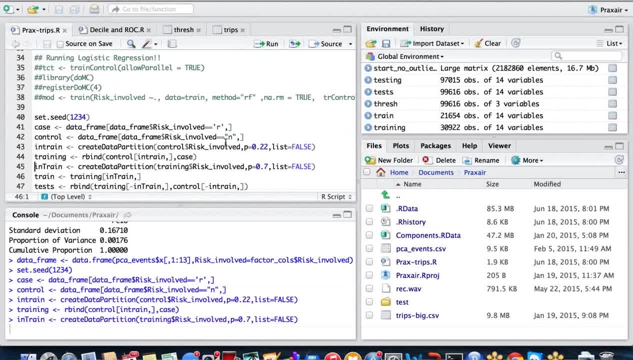 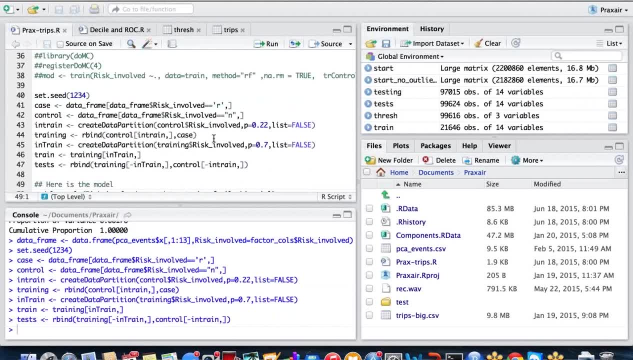 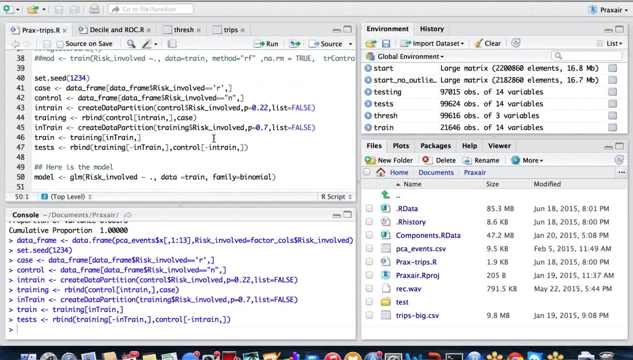 a training data set like this and now we create a testing data set. so basically, the trip data set that we used we divided into two parts. one was a training data set, the other was a testing data set. so we run our model on the training data set, which is the, the generalized linear model, and 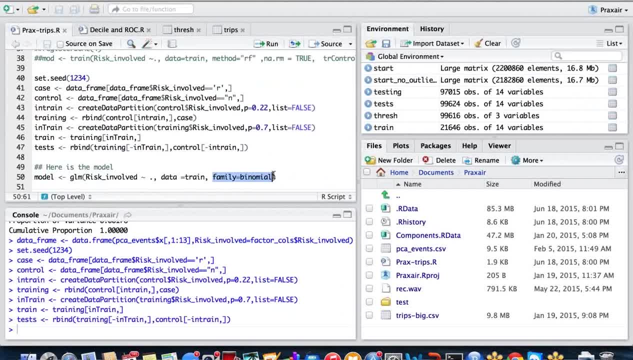 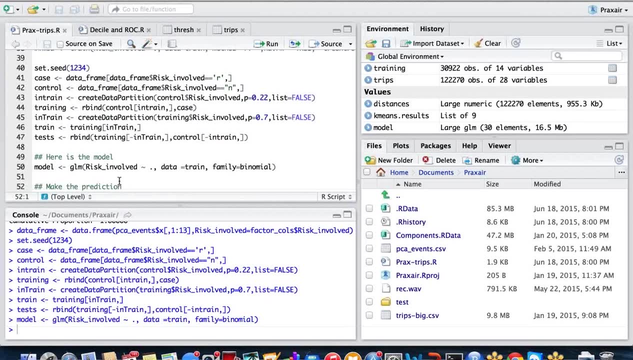 when I say family equals to binomial, it runs our logistic regression and I'm using data equals to train, to train my model. and here is the name of the model. name of the model is mo del, pretty, pretty fast. right now let's make some predictions. when I say type equals, response. 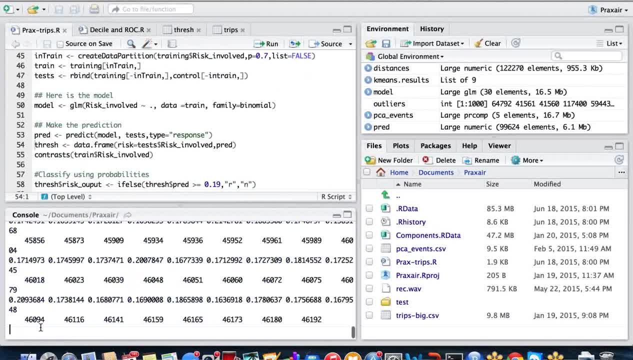 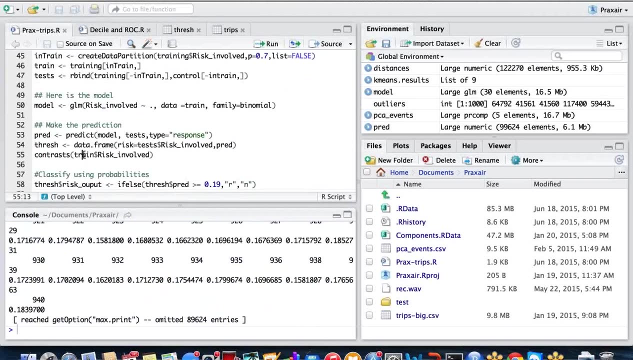 it's going to give me the probability. so let's see what does it give me thread? so it gives me some numbers: point one, seven, one, six one, blah, blah, blah, blah, blah. so basically, what it has given me is set of probabilities, okay for a particular event, but what probabilities? so when I say point 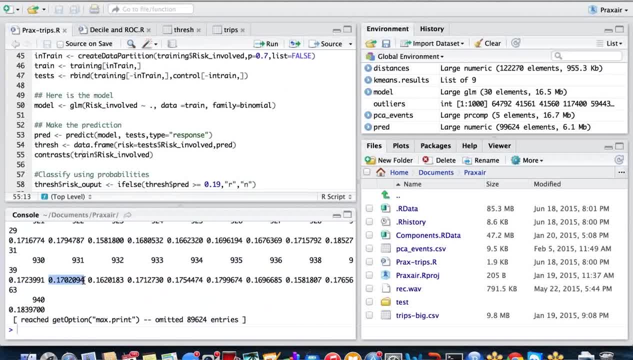 one seven. that means probability for an event is point one seven and the probability for the. so probability for one class is point one seven. so the probability of another class is 0.83. but see which probability is point one seven, corresponding to using this function called contrast. so it says: 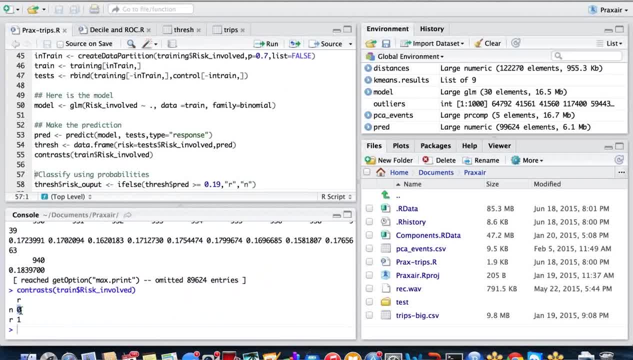 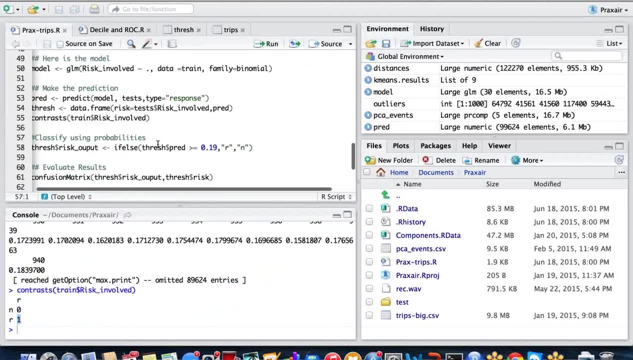 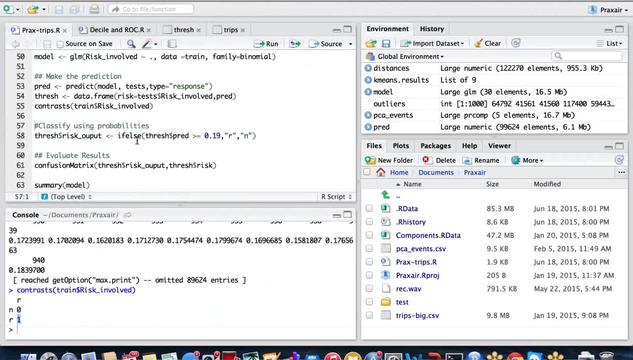 for risky the probability is is zero. so sorry, for non risky, probability zero and for risky the probability is one. so what so? so that means risk is the higher side and non risky is less, is like, is like on the lower side. so what I've taken is I've taken the threshold is greater than point one. 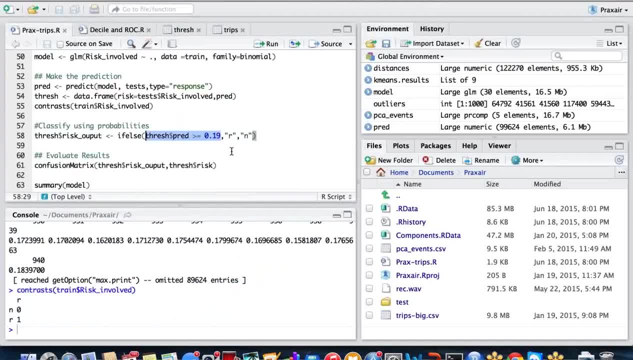 nine. so in cases where the probability value was greater than 0.19, I've marked those trips as risky and anything greater than 0.19, so less than 0.19, I've marked those as non-risky. so how did I get this numbers called 0.19? so basically I knew that the ratio of my my actual risky records. 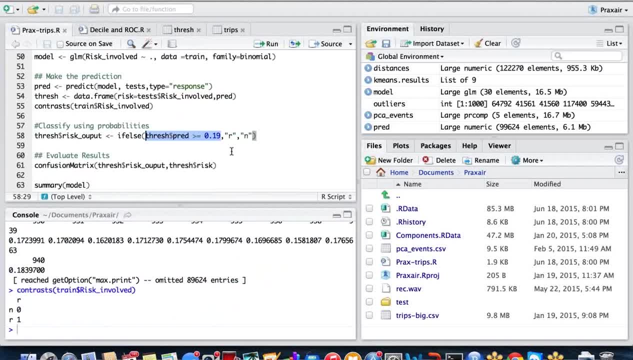 divided by my total records, was somewhere around 0.19. okay, now we create a confusion matrix to see what was my final prediction. okay, well, I get something like this: so out of so, six and five zero nine are the records which they got them said were non risky. 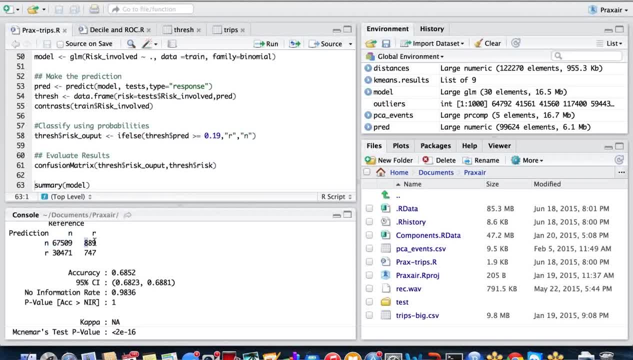 and they're actually non risky. eight, eight, nine were the records which the algorithm said were non risky but they were actually risky. then three, zero, four, seven, one other records which the algorithm said they are risky but they are not risky. and finally, seven, four, seven are the number. 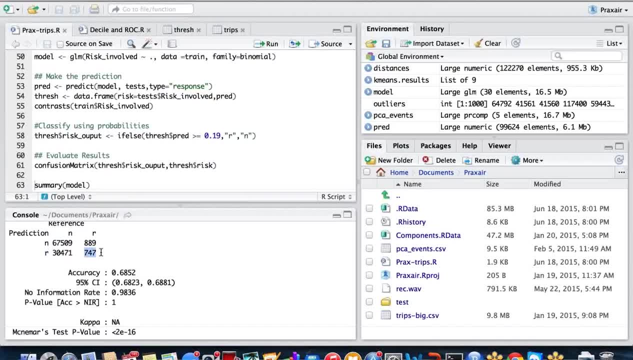 of events that were risky, and the algorithm also figured out that they were risky. okay, so, so that's interesting, isn't it? because our accuracy is like the total number: risky trips were eight, eighty nine plus seven, forty seven and the total accuracy is: isn't that great right? let's see what's the accuracy. 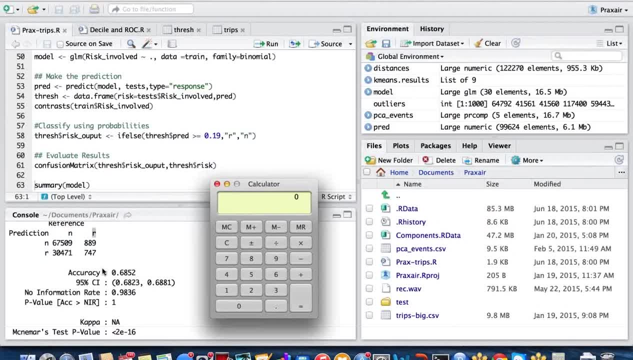 is so and figure out the accuracy, which is seven, four, seven divided by seven, four, seven and eight forty nine, which is somewhere around one, three, one, three, two, seven. so one, five, three, seven. so let's mark it a one, five, four, zero. whoops, or what? let me do it again: seven four, seven divided by one, five, four, zero. 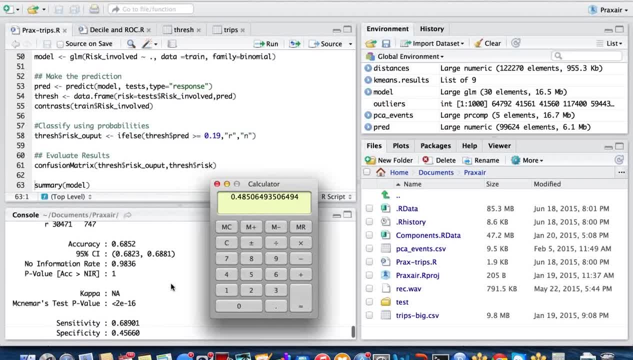 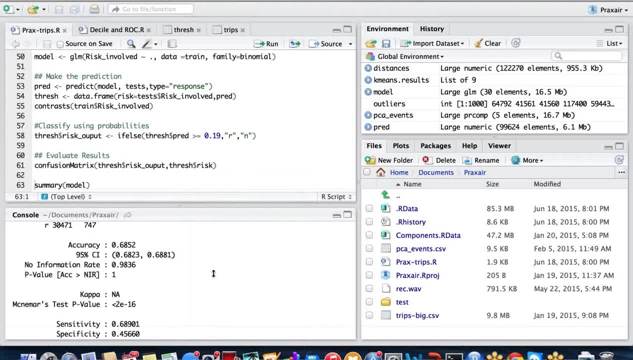 and we get an accuracy of one point four, eight. so is that a good accuracy? well, that's a mighty good accuracy if you look at it, because if you call certain trips that were not risky, but you call them risky, that's fine, because then you can take extra measures. but it's important that 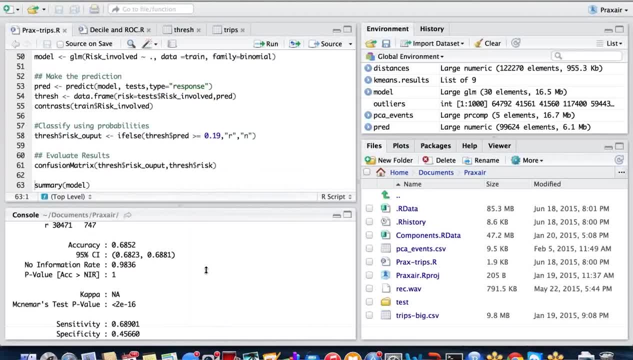 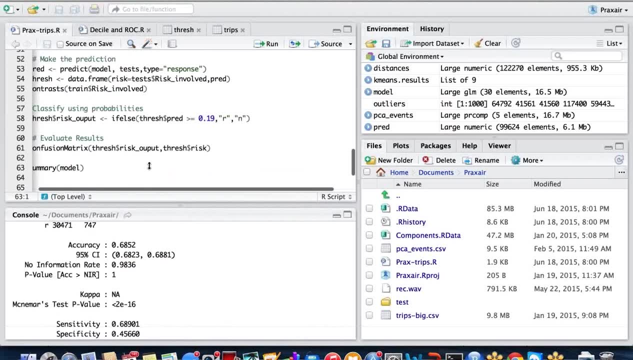 you are able to actually predict 50%, or somewhere near to 50%, of the trips that are actually risky, and you should be able to mark them as risky. so that's a pretty, that's a pretty lenient or pretty pretty acceptable accuracy rate. let's 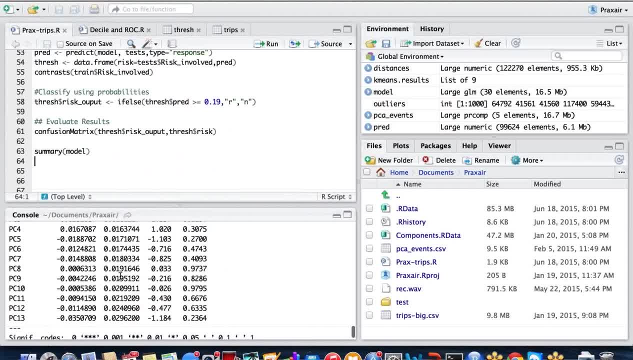 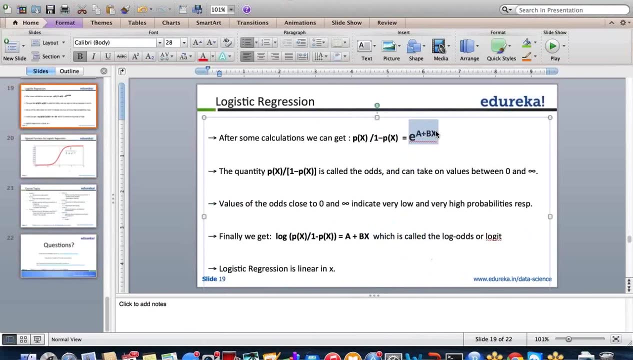 see the summary of the model. summary of the model is it used 13 columns, from PC 1 to PC 13, and these are coefficients. so these are nothing but the coefficient that we saw here. so these are those coefficients: a plus B, X. so a is, is the. 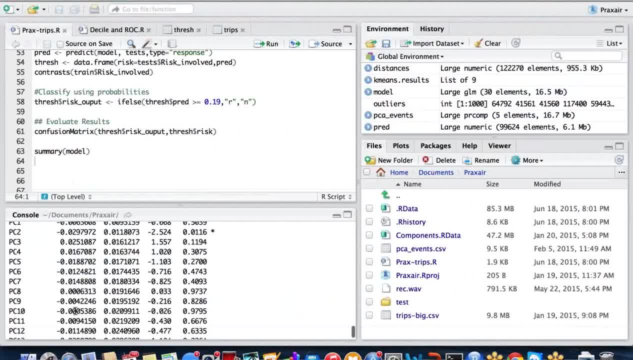 intercept, which is this and B. are these different, different variables? so it's like: minus one point five, four, six. one plus point zero zero six. minus point zero. zero six into X 1 minus point zero two nine into PC 2 minus point zero two five into PC 3 minus. 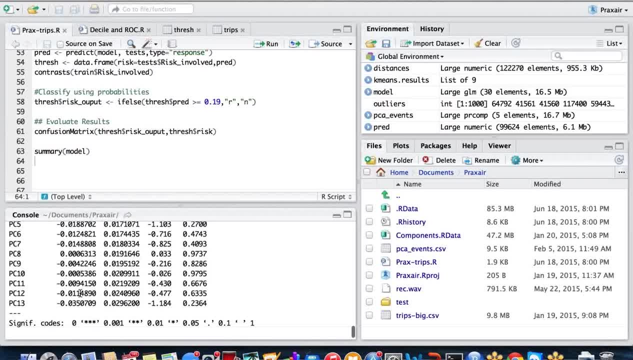 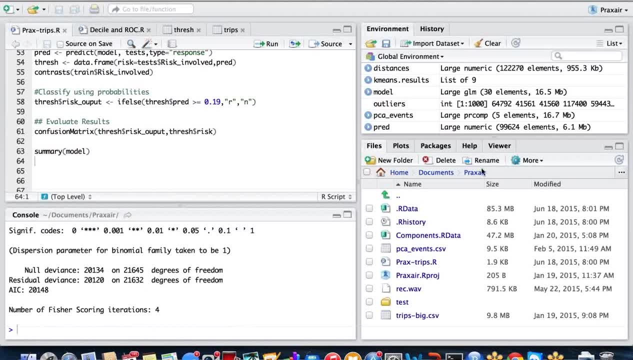 zero point zero one, six, seven into piece of four and so on, and that's how we construct your model. okay, fine then. so let's start with some questions, and you all can. you all can put up the questions now and let me see if I can answer those. 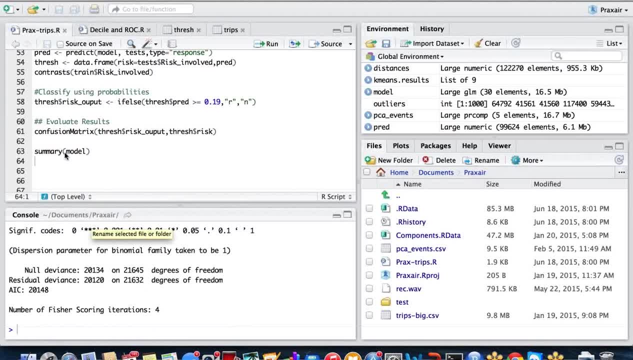 questions right now. okay, so they're mighty. I mean there plenty of questions that you guys have already asked. so what is KNN? KNN is your K nearest neighbors, but I've not used it. KNN basically figures out how are your neighbors doing so? for example, you got a. 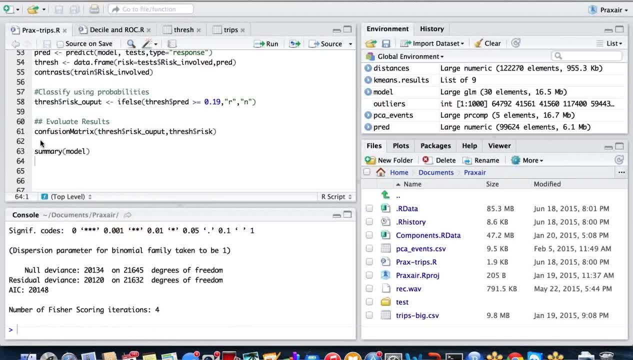 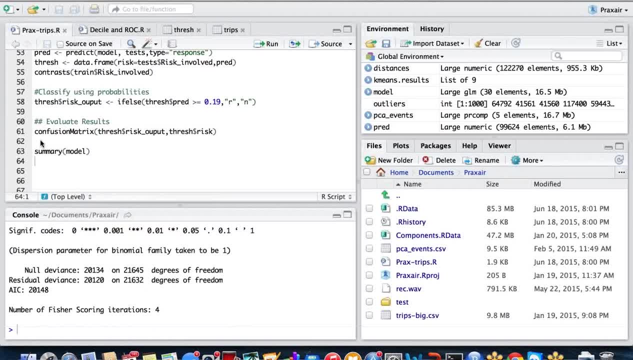 are. what is the output for those records? now that the question is: what is advantage of using audience Mahoud? well, r is, are is basically a these statutory modeling languages. language Mahaud is is running the statistical algorithm in parallel on hadob. okay, so well, they're advantage of. 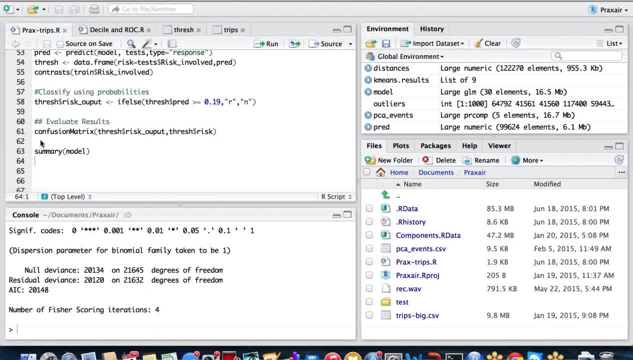 running art, RKằ� and most of the algorithms. my heart is still building up. it does not have the, the, the library, the, the advantage or the capability of running all those algorithms. I want to apply svm for machine learning, so do our. yes, of course, you can apply svm using a package called e1071. 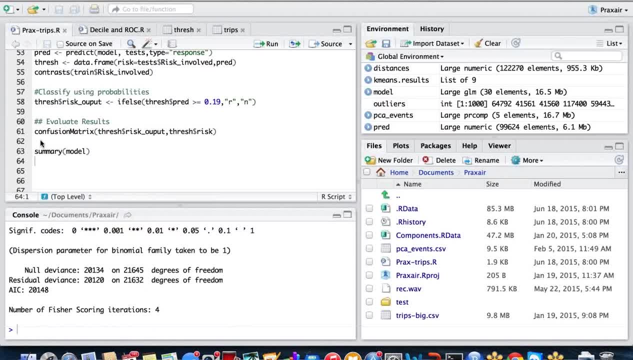 there's another package called current lab that you can use to run svm. we don't need to learn hadoop spark for a data scientist. well, it's not mandatory. I mean, it's not the primary skill set, but it's uh, now turning out to be a very important skill set. so the answer is that first master your. 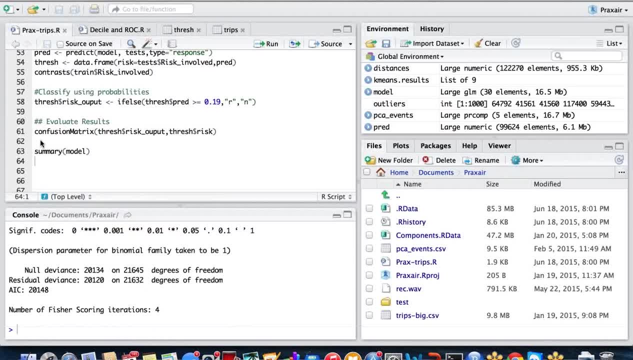 statistics and then you go for learning, for hadoop and spark. how do you decide? the threshold is 0.19. well, well, accuracy of 0.19. sorry, the. the threshold of 0.19 was based on the number of records that were there in in the training data set, which was like. so I had around 19,000 records. 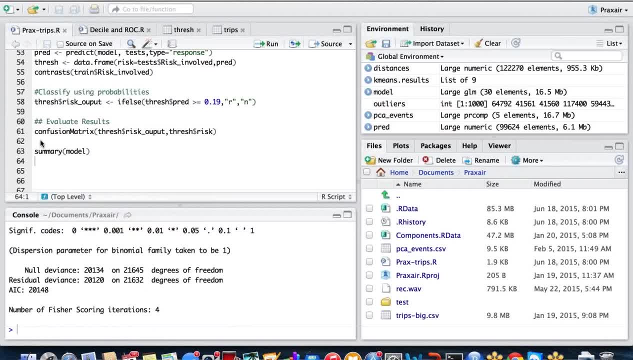 which were, uh, risky and rest of them were not risky. uh, how do you determine which attributes to include in a prediction? so that's a very good question, anand, uh, there's no direct answer to it. okay, there are multiple ways. so pc1 is one the the principal components that I used. there are 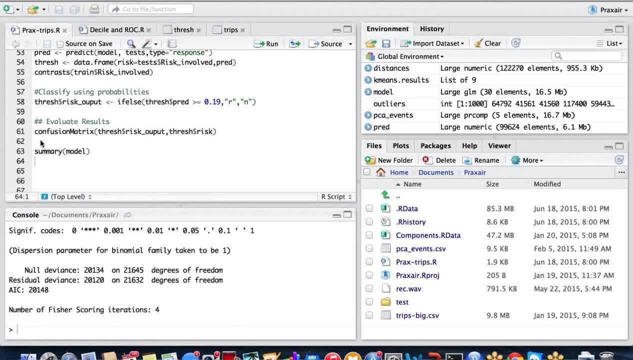 multiple other ways. when you find the correlations, you find which, uh, particular set of columns are more helpful, and the algorithms to do that. so, so it's one of the most important, important, uh, uh, important, uh uh aspect of machine learning, and this actually is the one that makes omar your entire model. how do we, why do we, normalize the 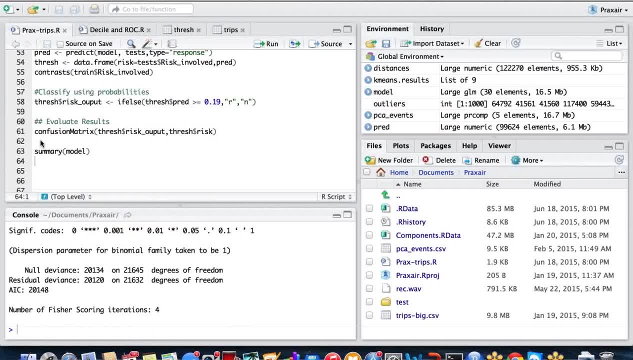 data. so we normalize the data because, uh, in k-means clustering, we figure out the distances between two. we got them two records. so basically, if let's say the features are salary per person and age of a person, okay, so let's say salary per person is ten thousand and age of a person is 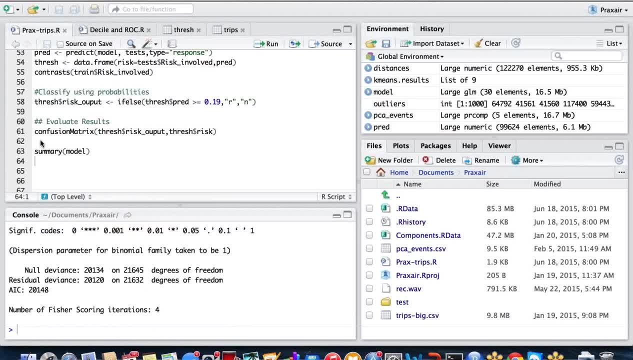 twenty, and there's others, another person with age is twenty thousand and salary is an age. sorry, salary is twenty thousand and age is twenty two. so the distance between these two guys are huge because you, when you, when you, when you find the distance that's twenty thousand minus one thousand. 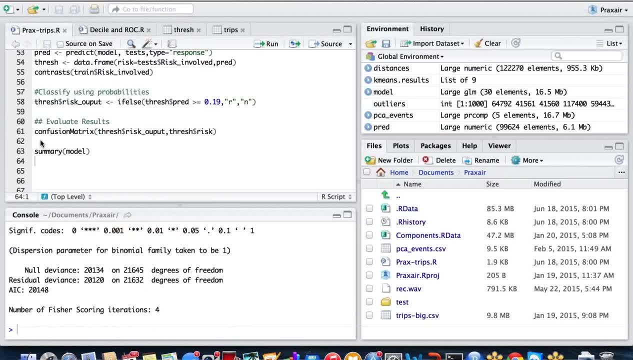 whole square plus twenty two minus two, twenty whole square under root. so basically, your age does not help in the distance, it's majorly the salary which is figuring out the distance. so you need to normalize the data set so that each algorithm, each column has, uh say, 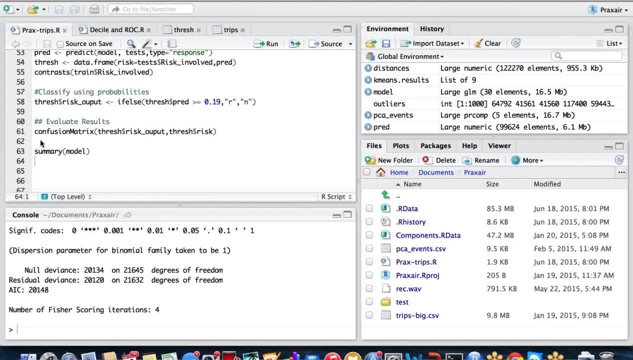 has a value, has a proposition to make in the final model when to choose logistic relations. also, in which languages language, the machine algorithm, certain. so see in r the algorithms are mostly written r only, but the underlying uh language is c plus plus. well, uh, we there are. 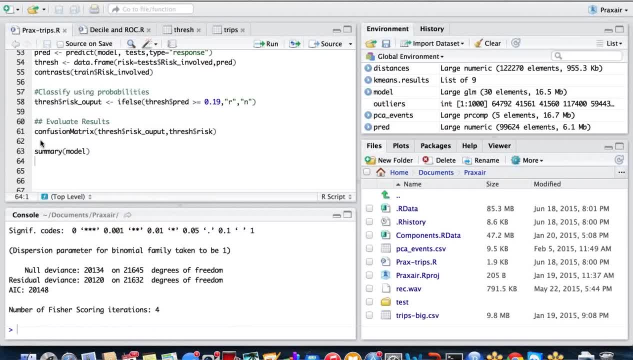 certain libraries that work with java. they are certain that work with c plus plus. but i majorly use r and python. so r and python are the most most you know widely used uh languages. for for machine learning to choose logistic regression means in which class case i should. okay, let me just read it completely. 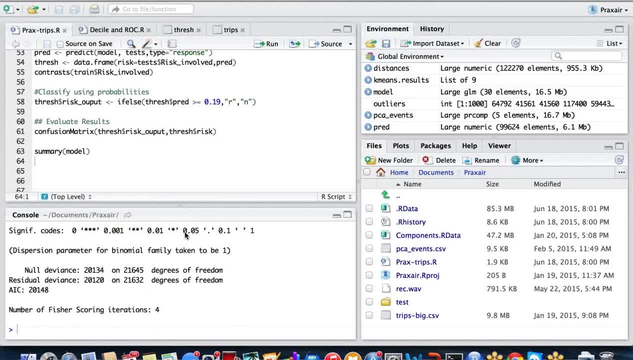 okay, so when? to choose the elastic relation means, in which case i should choose the oscillation prediction either. this method like random forest. see, uh, there is no right answer to it again, okay, you, there are certain properties of a logic regression which makes it better than, uh, random first. so, logistic regression based on maximum likelihood, whereas random forest is based 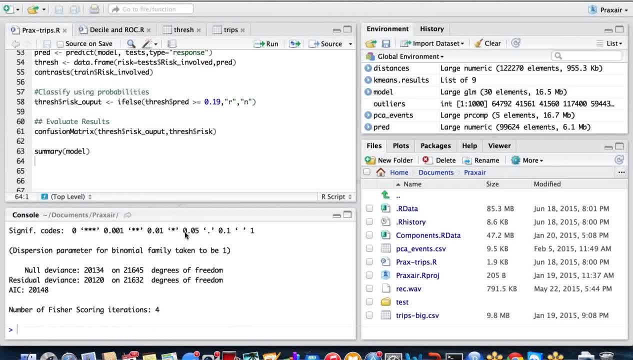 on the vote based on the decision trees: okay, so it's actually question. it's basically uh, a question when you, if let's say, if you can do things well with a linear regression or a linear classifier, then i would go for a logistic regression, but if things, my data, is linearly, 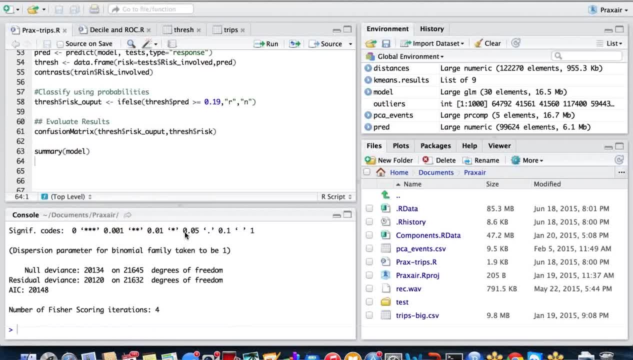 not separable, then i would go. i would want to go for random forest or svm or any ensemble. how can you say accuracy is less than 0.5 is pretty good accuracy, so it's effective if you see deep right. no, that's Lakshman, so Lakshman if you see that the algorithm wait if you. 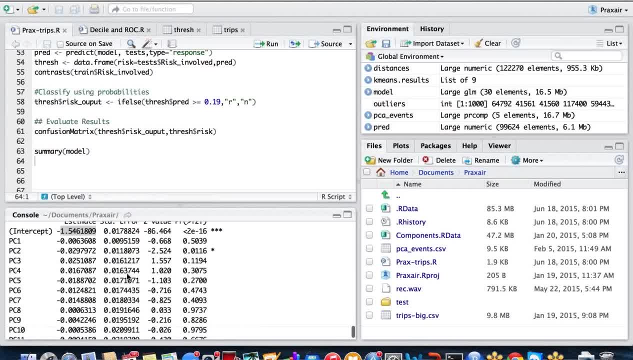 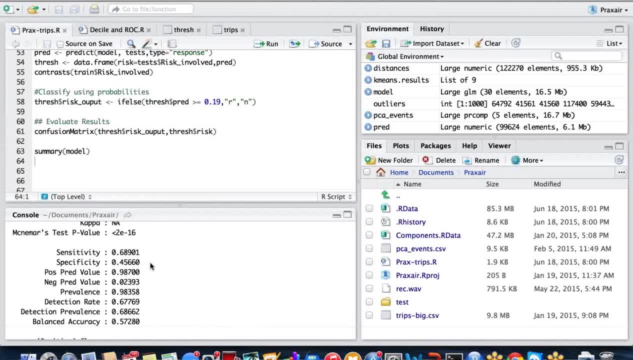 see, my accuracy actually is not 0.45, it's actually the specificity. okay, so specificity is like 0.45. okay, so someone is raising hand, so what do it? okay, let me go back to the questions. so the accuracy is 0.45 or 0.46, whatever that means, out of all the ones that were risky. 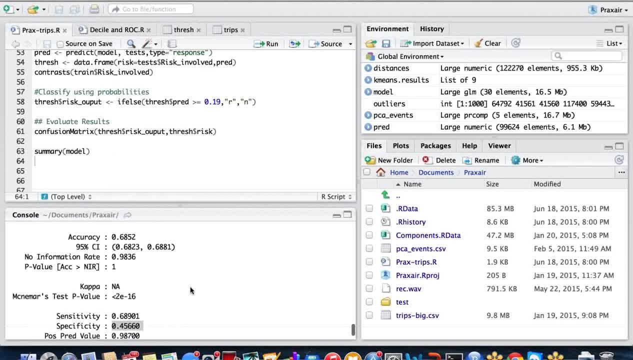 0.45 is a 45%. with 45% accuracy I was able to figure out the risky trips. my overall accuracy is 0.68. okay, it is just the specific accuracy, or the specificity as we call it, which means if, let's say, if I, if I was running. 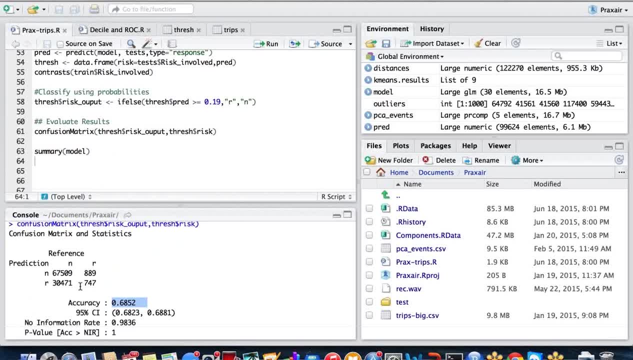 a random classifier. okay, so a random classifier will give me a very low space accuracy, my sorry specificity, my accuracy would probably go up. maybe it would be 70 or 80%. or let's say: I call everything is non risky. if I call everything is non risky, I am bound to have 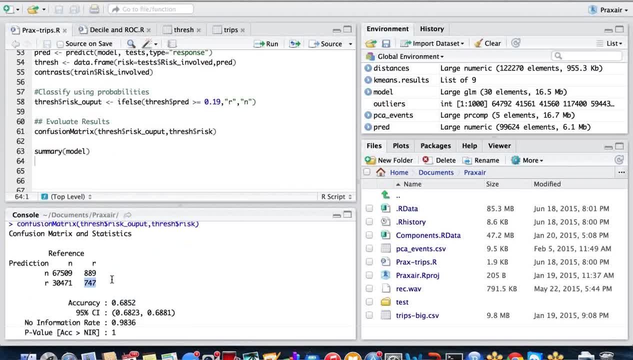 accuracy of 80%, but my specificity would be 0. okay, okay. so my specificity is something that I want to bank on. I want to ensure that I do a good job as compared to a random classifier. so a random classifier here will not go beyond. 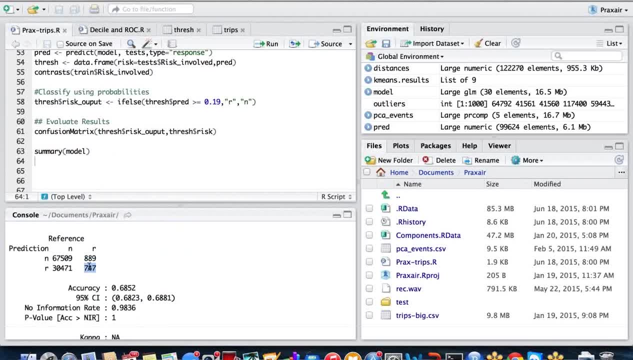 5%. okay, of course, if you've not. if you, if you solve these kinds of problem more, you'll understand why and where the accuracy beyond 0.5 or somewhere close to 0.5 is really good, because that's specificity and that's not accuracy. so let's say, let's say you got a. 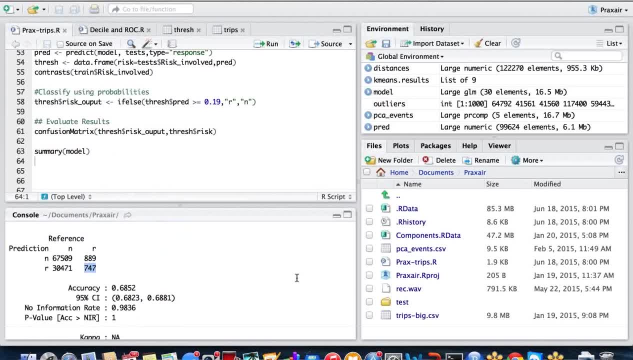 person on our web page and you want to figure out whether you have a specificity or not. so you want to figure out whether this person is going to click on my ad or not. now I already know that out of thousand, only one click on it, so I call this guy also has as not clicking. 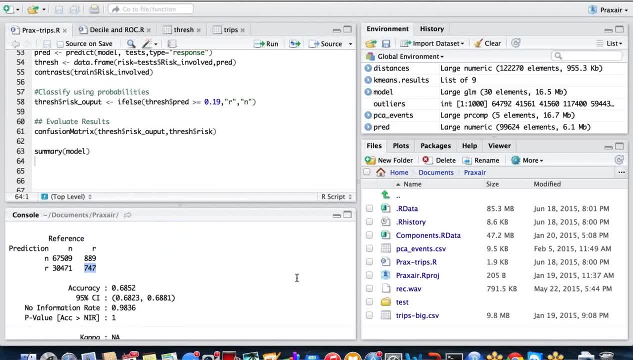 and let's say there were ten thousand other guys and I called all them as as not going to see click on my ad. so out of this ten thousand expected is like hundred people will actually click on. ten people will click on my ad, but since I called every one of them as someone, 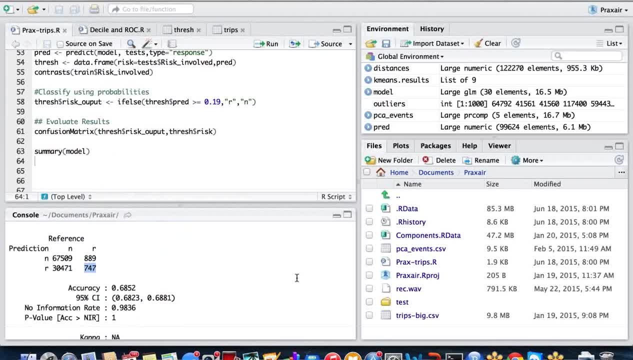 who's not going to visit my ad. Then I also accurately classified nine thousand nine and ninety guys, because you're not clicking. so my accuracy is ninety nine point nine, but that's not what I'm looking at. I want to figure out: out of those ten, how many can I, can I could you figure out, and if I can, accurately? 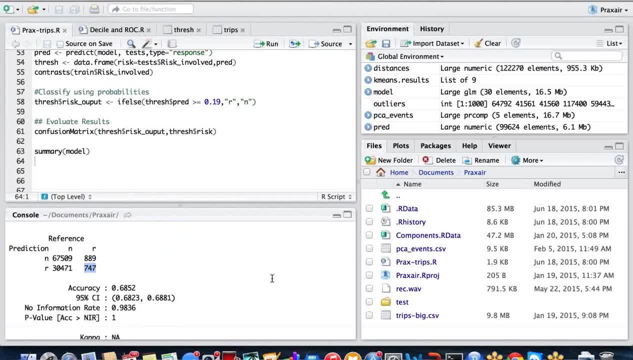 figure out four, then I'm, then I'm, I'm done, five or six, whatever, then I'm not doing bad. okay, how can you say okay, how to choose best customer, because we've got plenty? I think I've already answered that. you need to see the data set. 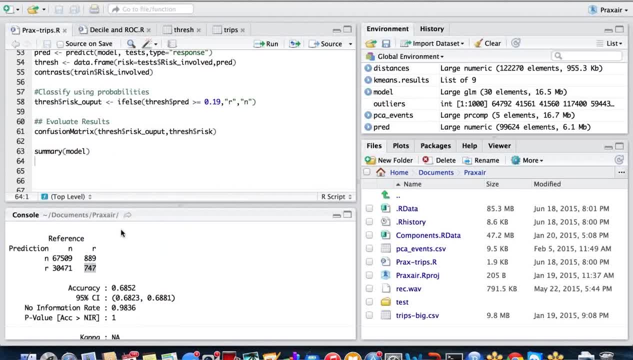 Your data behavior. can I have two decision attributes? I don't understand this question, but I think you meant: can we have more than two decision attributes? can we have more than? can we have more than two classes? the answer is yes, absolutely, we can have more than two. 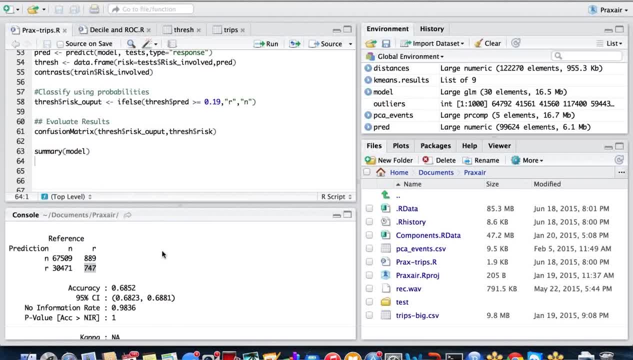 classes, how this algorithmic algorithm can help us create the accuracy while we trade. what is that trade? basically, I use regression model to find out the possible higher and medium minimum level of The stock, but most of the time it's got beyond those levels, which are got three different. 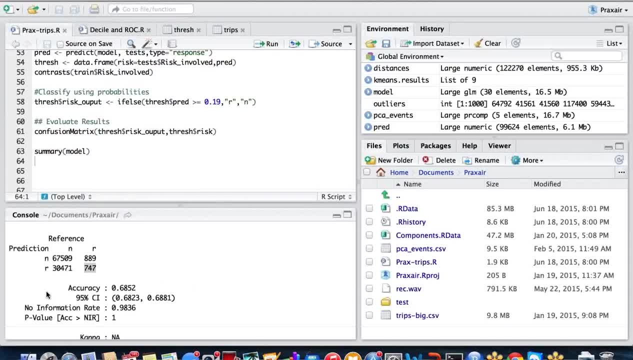 obviously so. see, it's not that easy. so you need to find either the most complex of the algorithms- and that's why the, the, the algorithmic trading guys, have paid really high, really high, and, and, and, and, to get to the accuracy where you figure out the possible higher in the. 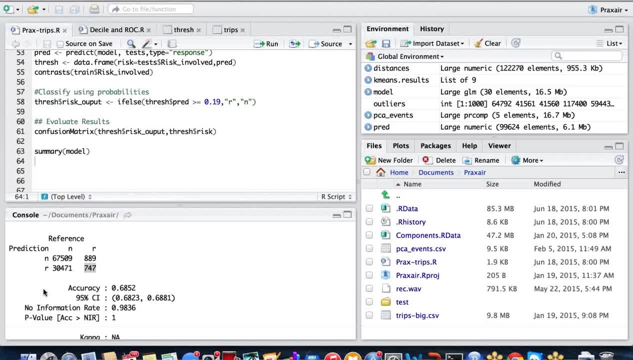 minimum value of a stock. it's not going to be easy, because we could do that. you'll be a millionaire, right? so the answer is Is: Is yes, the algorithm can help, but how exactly can help? well, there are thousands of things that actually constitute that entire model and not just the algorithm. we should know. 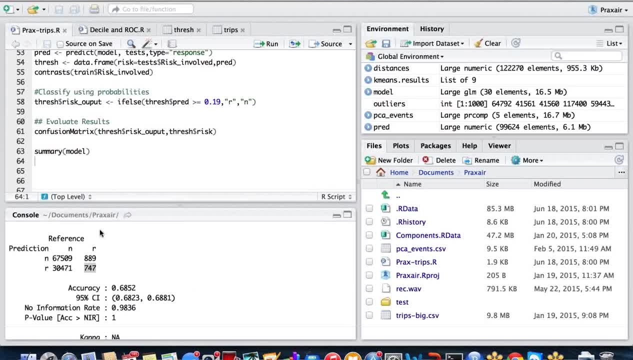 how to spark for data scientist. I think I've already answered that question. any more questions. we'll wait for another couple of minutes and then we'll close off this webinar. questions anyone so? I've already answered this question. We know you need to learn, in case I've been so. the question is that: do we need to learn? 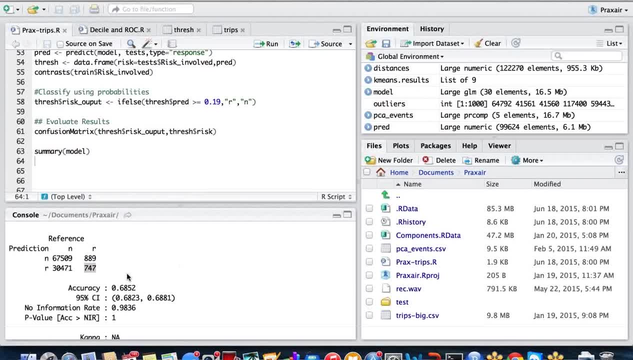 how to spark. see, it's not the primary skill, again, it's the second set of skills that you need to acquire. but do we need to? the answer is yes, we need to. eventually, not on the first, on the face of it, the primary skill set of a data scientist, one, as I've already mentioned. 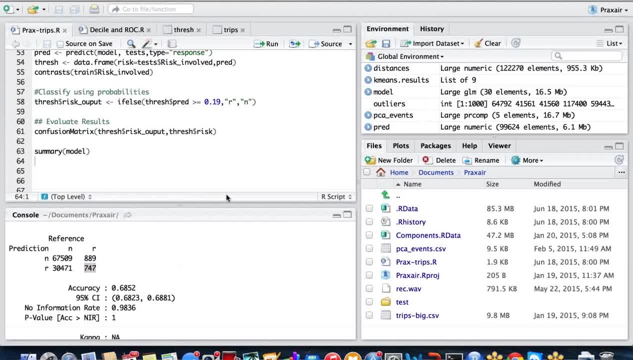 in statistics. you need to know that statistics, you need to know the math behind the algorithms. because we don't know the math then you're not able to model those algorithms accurately. because some algorithm do specifically good with specific kind of data sets for a specific kind of problems. so that statistics, second is either our Python, I would say. I would say: 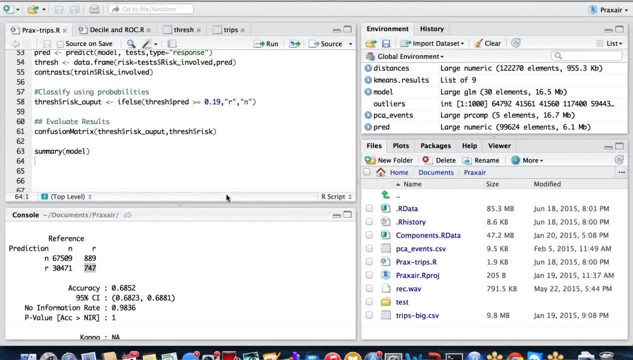 you, you do, you go for. both are in Python. that has to be the eventual goal, but you can start with one of them. third is a do pen and spark and all that For, for, for power processing, and then you should also have a good creative or a understanding. 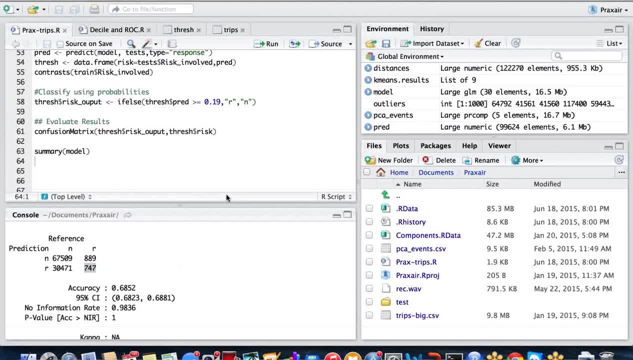 of the visualization part. you can learn D3 or you can do it in R. also another question which is: as are better? or says I can't answer that question because says if I say our size going to, you know I is going to assess, going to hit on me, but R is open source, it's pretty. 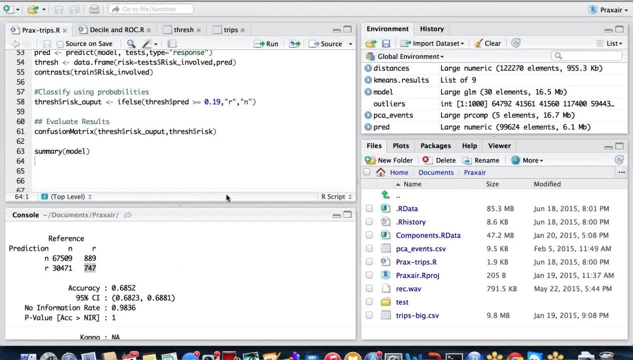 handy and it's. it's pretty cheap, Even with The corporate version and it has got and you can do the most complex. I know we can run most the most complex about them, also in our in size you can still do that. but says is is now confined to industry analytics and does move beyond the integration or GLMs I've 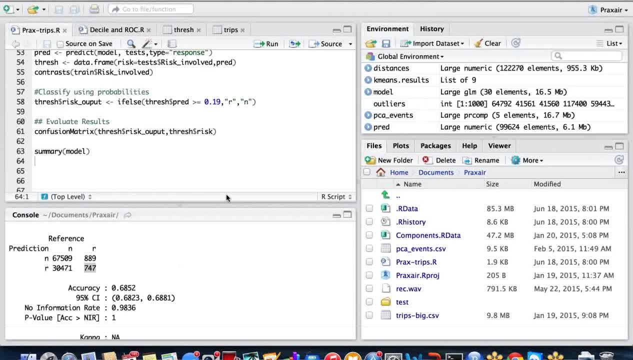 not used. I know for severance, as how would we should be leader aggression? it's like how would we should be in grammar if you want to speak English. integration is a must because it's simple. And Because it's simple it does not mean it's, it's not required. because it's simple, I would. 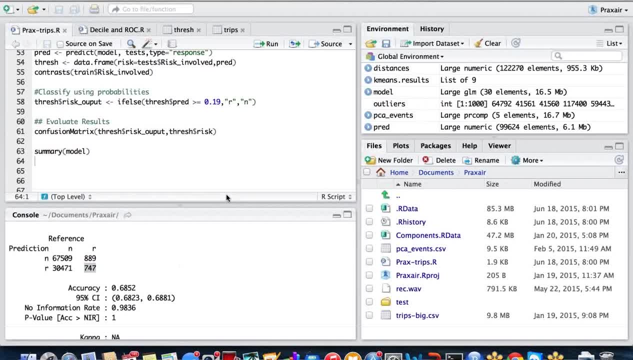 say it's really important because that helps you understand the rest of the algorithms. plus, the first step where I saw any problem is actually put up a linear regression on that data. So, guys, we are done with the webinar. thank you so much for joining in. I hope this this. 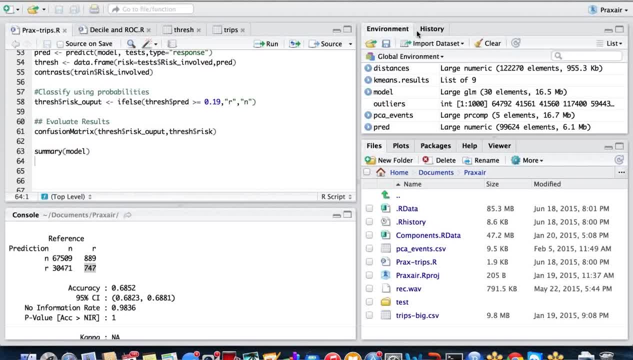 was informative and helpful for you guys. thank you so much for joining. bye, bye. 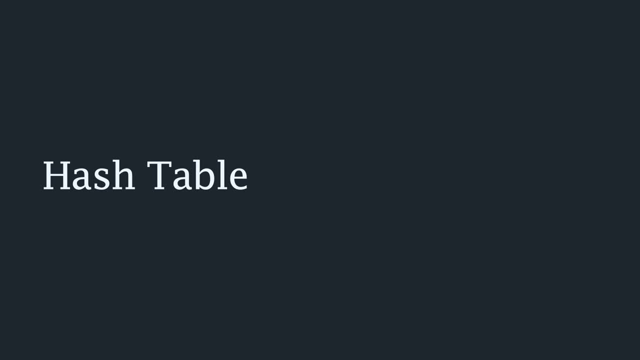 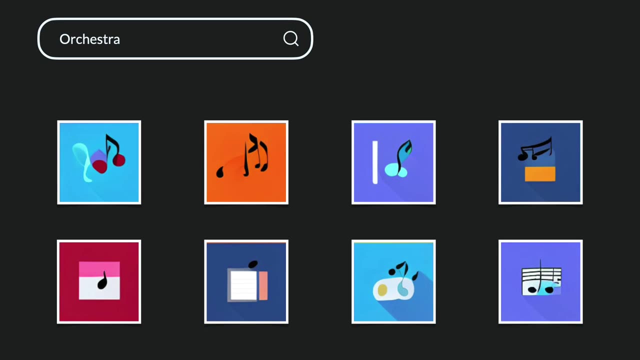 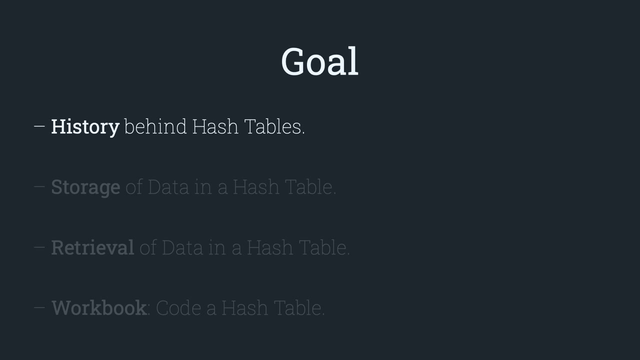 The hash table is a fundamental data structure in computer science. If you've ever wondered how search engines can find results so quickly, it is all thanks to the hash table data structure. First we will discuss the history behind hash tables and then we will explore the. 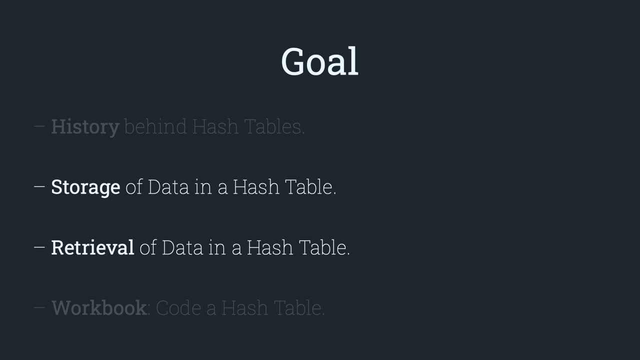 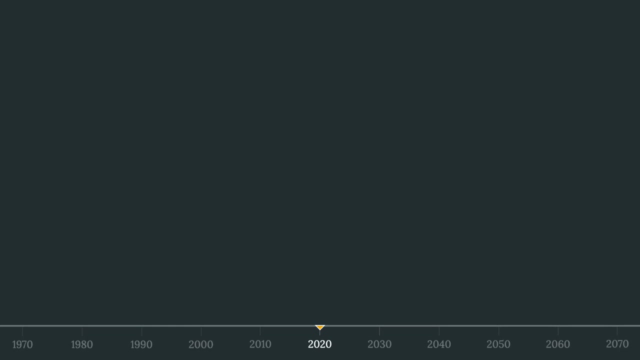 internal workings of a hash table, in terms of how they store data as well as how they retrieve it, And once you learn the fundamentals, I will provide you with a workbook where you can practice coding your own hash table. We will begin with some historical background, because we cannot discuss hash tables without